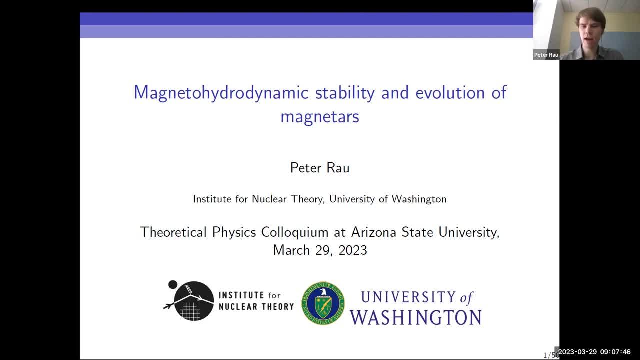 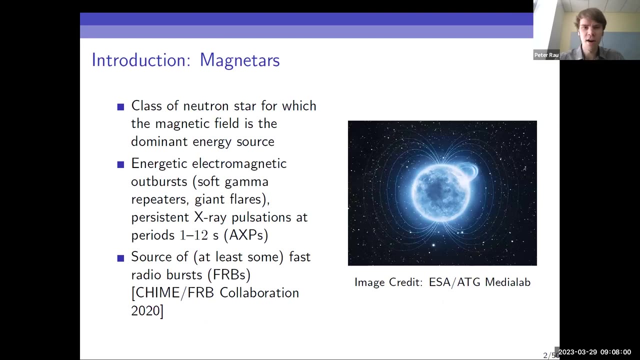 All right, thank you for that nice introduction, Igor. So yeah, I'm going to be talking about a series of papers and some ongoing work I've been doing on MHG, stability and evolution of magnetars. So you know, to go to the basics, you know what is a magnetar. It is a class of neutron star for which the magnetic field is the dominant energy source powering its electromagnetic emission. 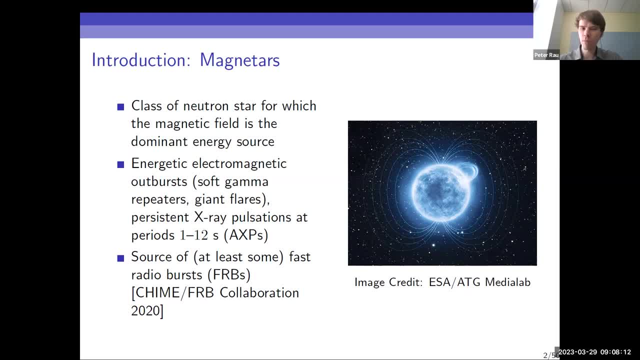 So this should be contrasted with, you know, more typical radio pulsars, for which it's the rotation which is powering the electromagnetic emission. So so magnetars are mainly distinguished by their energetic electromagnetic outbursts or their particular kind of periodic X-ray emission. 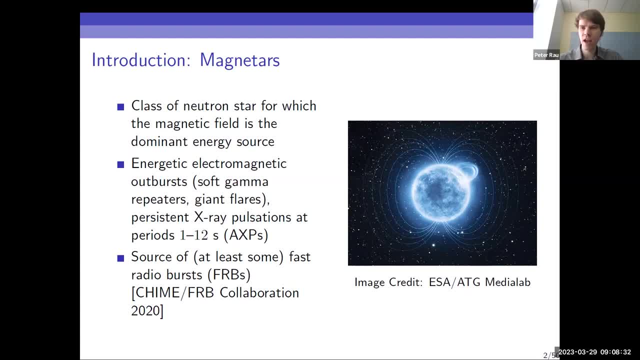 So these energetic outbursts are classified as soft gamma repeaters or giant flares, Soft gamma repeaters being repeating but not periodic bursts of, you know, soft gamma rays and giant flares being much rarer but much more luminous events of gamma-ray emission. and additionally, magnetars are known to emit pulsating X-rays. 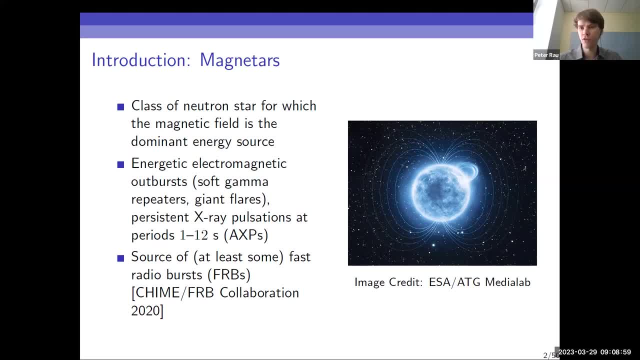 at long periods relative to the rotation rates of most neutron stars. so these are of order 1 to 12 seconds or so, and their spectral characteristics are quite different from other types of neutron stars which are emitting X-rays, most of which are accreting, and so 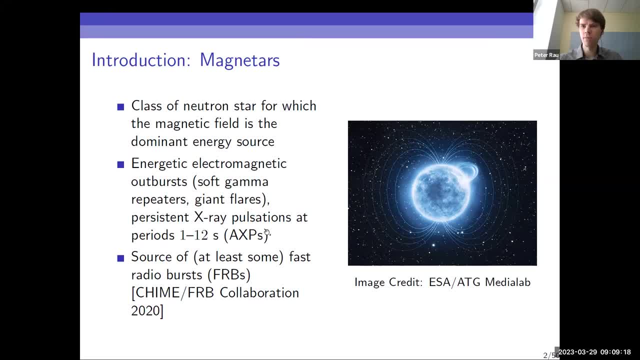 these X-ray emissions got them termed anomalous X-ray pulsars. Additionally, magnetars are believed to be the source of at least some fast radio bursts, which are sort of bursts of radio waves in the gigahertz range which are lasting a few milliseconds but which are 10 to the 12 or 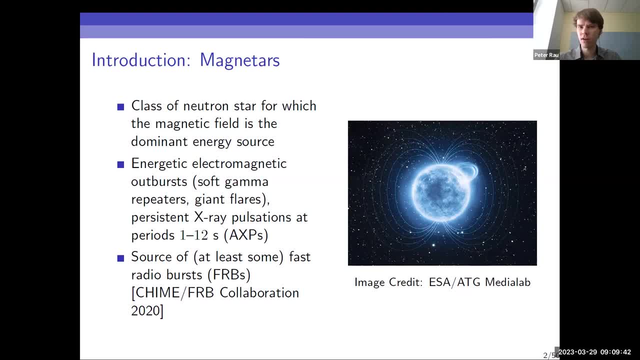 so times more luminous than the radio signals from X-ray- sorry, from radio pulsars. And we know that FRBs come from magnetars, or at least some of them do, because of a localized FRB originating from a galactic magnetar. so that was measured in 2020 by the CHIME-FRB collaboration. 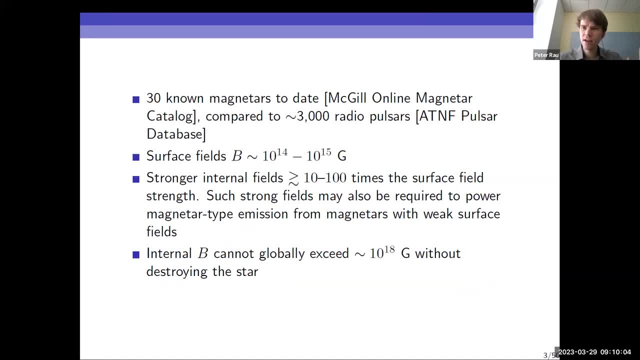 So there are about 30 known magnetars to date. compared with, you know the much more numerous radio pulsars. We know about 3,000 of those. That doesn't necessarily mean that the ratio of magnetars to normal, like radio pulsars, is actually this large. It's just that. 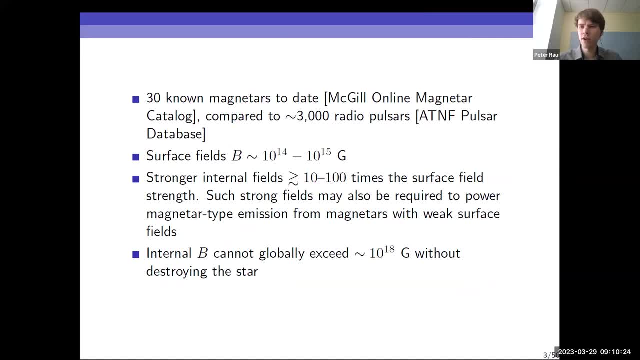 we haven't been able to measure many of the magnetars because they tend to have shorter lifetimes than radio pulsars. They burn brighter but also, you know, are more ephemeral, essentially, And so I've been talking about this magnetic field a bit. How strong are these? 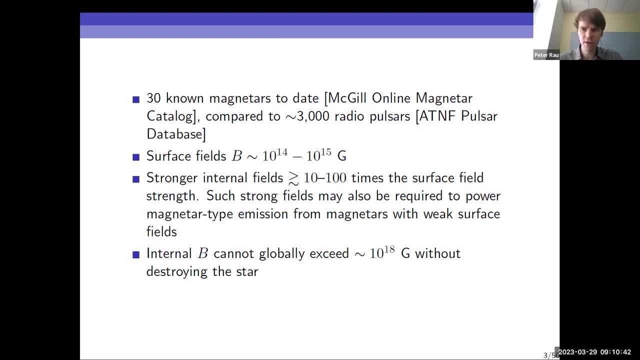 magnetic fields At the surface. they're typically of order 10 to the 14 or 10 to the 15 gauss for magnetar. That's, you know, one of the things that we've been talking about. And then you know we've. 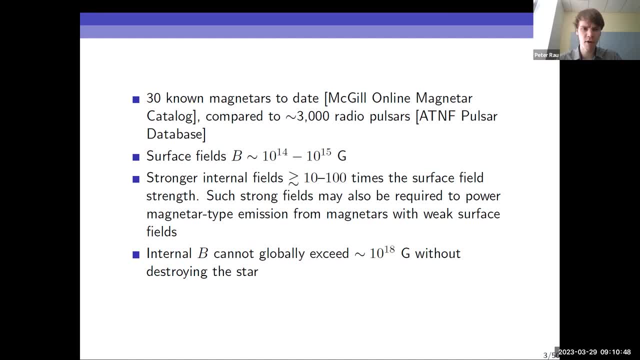 been talking about the magnetic field as being 100 to 1,000 times stronger than the typical surface fields of a radio pulsar, And the internal fields are believed to be even stronger. If you imagine the field was modeled as a dipole, it should fall off with radius, so of course you'd expect the 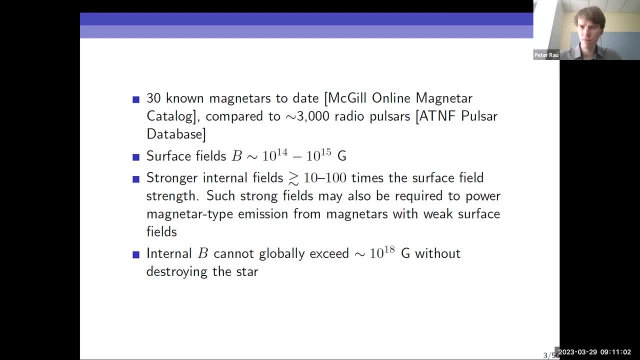 field to be stronger inside. But additionally, there are types of magnetars which have been observed which have weaker surface fields than those shown here, but still emit these energetic electromagnetic outbursts, And so it's believed that there has to be a buried magnetic field. 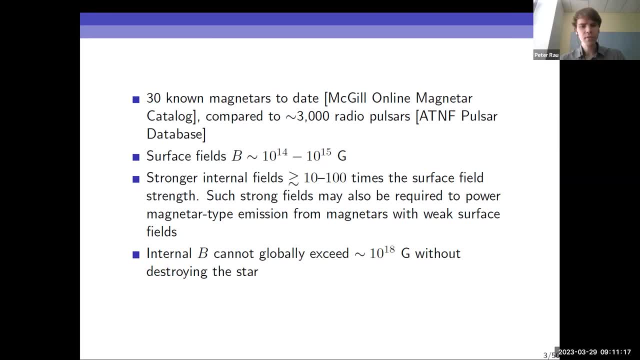 which is powering those Types of outbursts. But the magnetic field has sort of an upper limit and that if you exceed around 10 to the 18 gauss at a global scale, so like the average field inside was that strong, the magnetic energy would overpower the gravitational binding energy of the star. 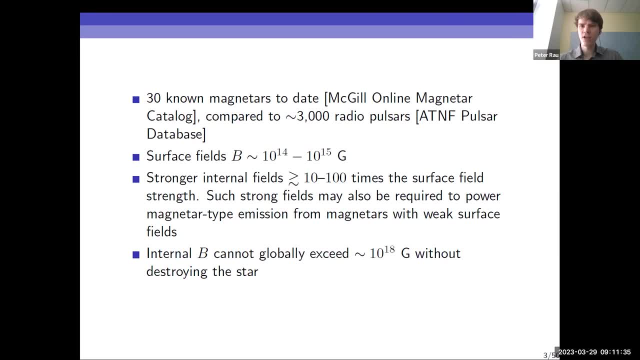 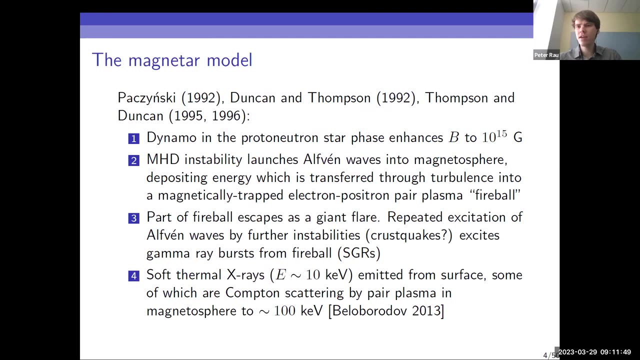 and it could not exist. So essentially you have a sort of maximum that you could have as the like globally average field strength. Locally it could exceed that, but not at like a sort of average value. So the idea of magnetars as this concept which unifies these, 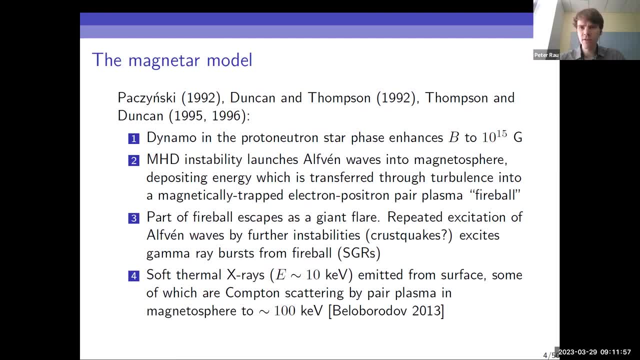 different emission mechanisms. you know the unified source for them was developed in the 1990s, after these emission mechanisms had been observed starting from the late 1970s. And it's principally, and the details of this were worked out in a series of papers by Duncan and Thompson. 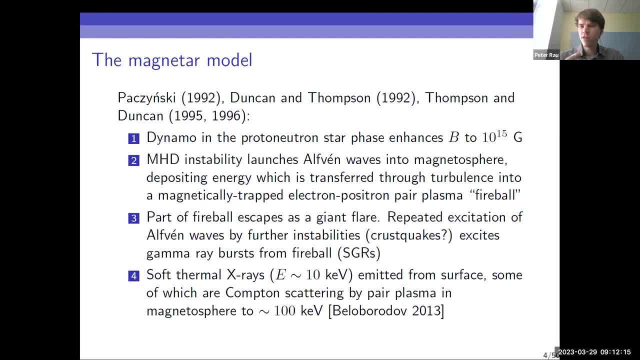 And so the idea is that once the neutron star is born after a core-clop supernova, it's much hotter and the motions of it you can have these different instabilities which develop. So the initial model was a convective instability, but also the magneto-rotational instability can also be active. 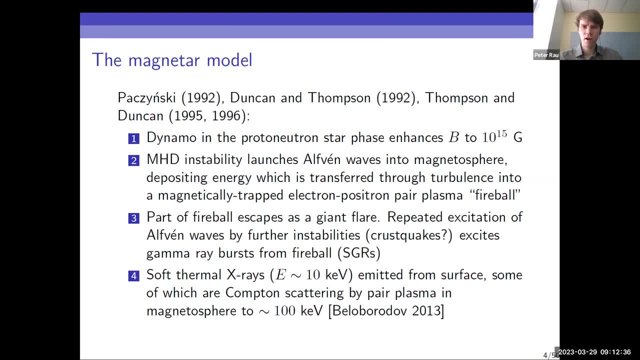 And the idea is that these instabilities grow. You have a turbulent cascade of energy to small scales and that acts as a turbulent dynamo to enhance some energy And even though you have the initial seed magnetic field, up to values, of say, 10 to the 15. 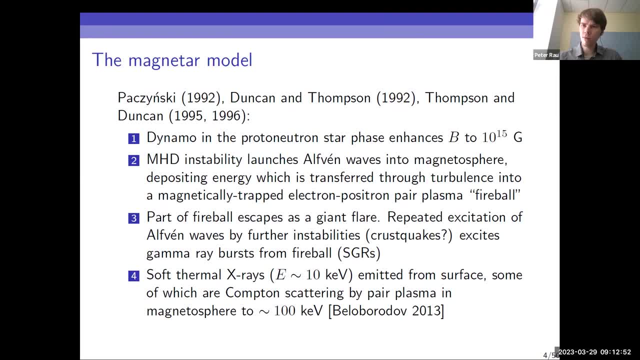 Gauss. and then, once the star cools somewhat, you're left with a magnetar, you know, neutron star of typical neutron star sizes, with a much stronger magnetic field. And then something happens later on, some sort of MHD instability inside the star which launches Alfvén waves. These are a type of 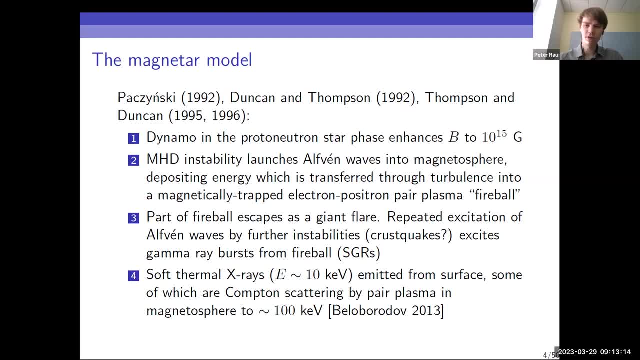 oscillation which moves along the magnetic field lines, But the oscillation is still very strong, perpendicular to them, and the oscillation carries energy into the magnetosphere surrounding the star deposits that energy, and that energy is transferred through turbulence into what's known as a magnetically trapped electron positron pair- plasma fireball. part of this. 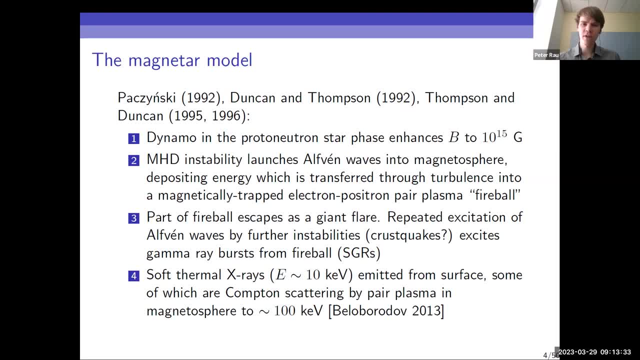 fireball can escape the magnetosphere and that would be observed as a giant flare. but you still have this pair plasma fireball being trapped by the strong magnetic field and if you had later maybe smaller scale excitations of that, perhaps caused by a quake of the crust which could occur, 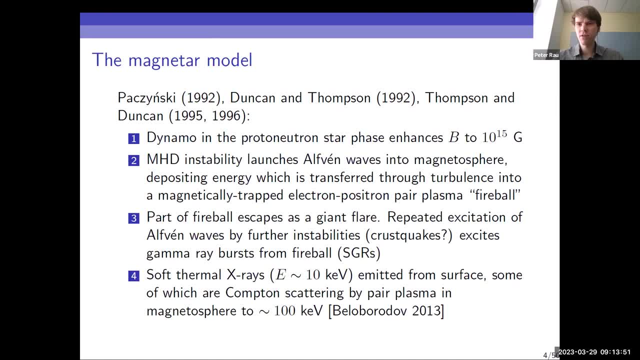 if you have a buildup of magnetic stresses, or stresses due to the rotation rate decreasing, that causes the crust to undergo failures and because you have field lines being anchored to that crust, they will be, you know, shaken and they'll excite these waves that deposit more energy into this fireball, launching smaller. 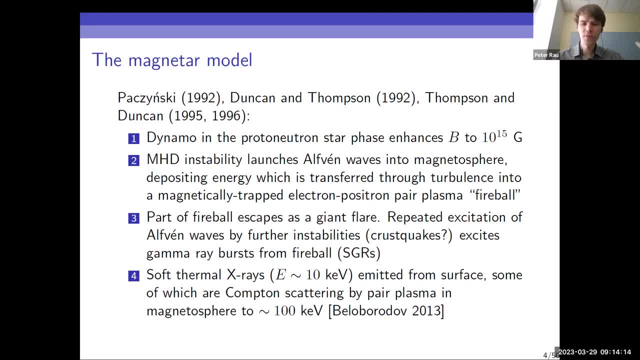 energy into the star and then you have the first of gamma rays and so that would be observed as the soft gamma repeaters. additionally, because these stars have these very strong magnetic fields and you have charged particles following the magnetic fields and colliding with the surface, you have a soft thermal x-ray emission from the surface. but because you have these paraplasmas, 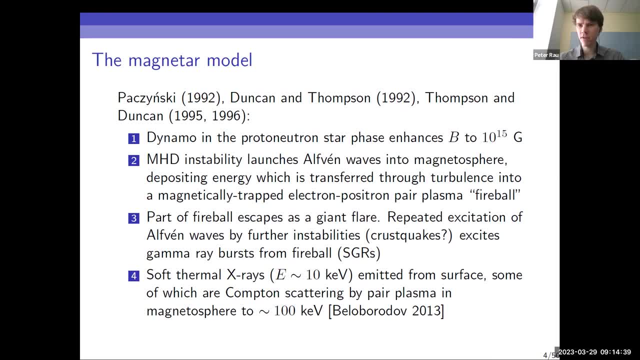 trapped in the magnetosphere. some of those softer x-ray photons will be upscattered by the magnetosphere, and so you can see here that we have a kind of a different type of energy emission from the magnetosphere to sort of the highest energies seen in the 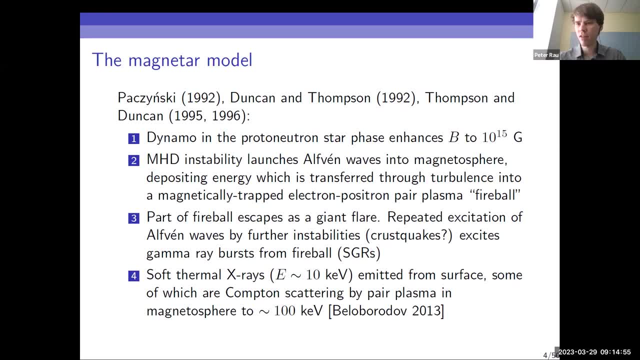 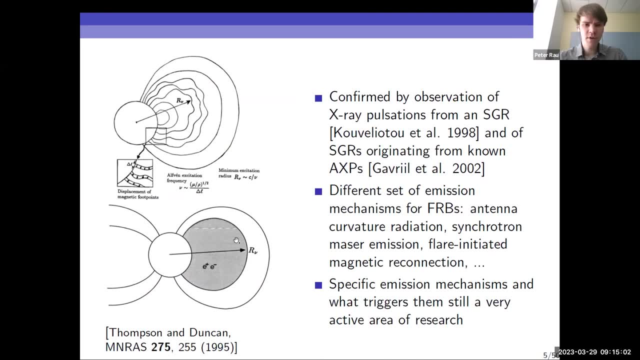 spectra of anomalous x-ray pulsars and so that this model in total explains the different emission mechanisms, at least for the three types of classical emission from magnetars. so again, this is. these sorts of aspects are illustrated on the left here. so the paraplasma fireball and then the excitation of the alphane waves in the magnetosphere. 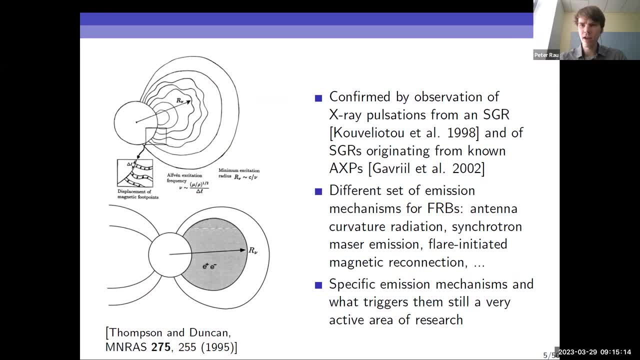 this is an example of the model of a soft gamma repeater that was created by making observations of x-ray pulsations from a known sgr and then observing a softgam repeater from a known anomalous x-ray pulsar, and so this sort of made us believe that this model was correct, that these 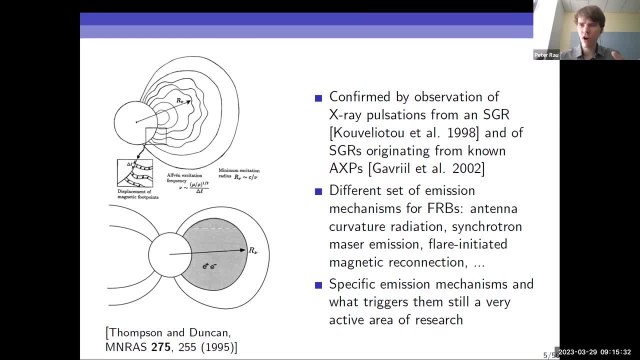 phenomena all came from the same objects with very strong magnetic fields. and the magnetic field needs to be quite strong because you need to be able to power repeated events. it can't just be something which is one-off because we know that. you know sgr is do repeat. 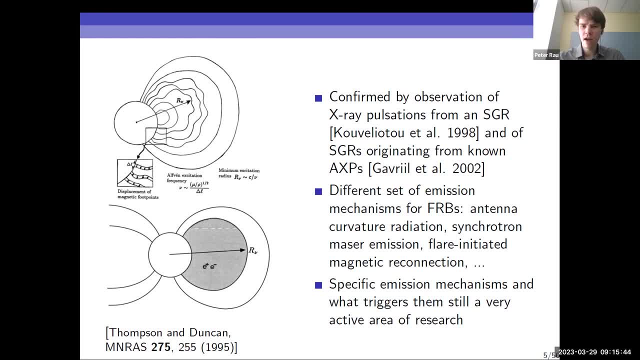 There are an entirely different set of mechanisms explaining fast radio bursts, which also invoke the storm magnetic field. I'm not going to go into those in any detail but this is a very active topic of research, very interesting to follow, Many different reasons to favor different models over the other, but it's still something which is hotly contested. 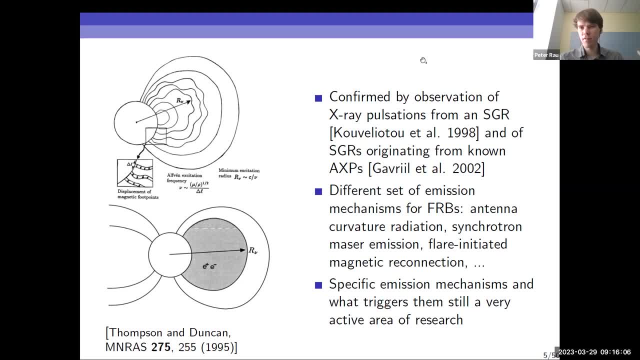 But one thing to notice: that the specific emission mechanisms in general, like a lot of these models, there's still reasons to put some doubt in. There's still reasons to doubt them exactly And there's still questions about exactly what is triggering these emission mechanisms. 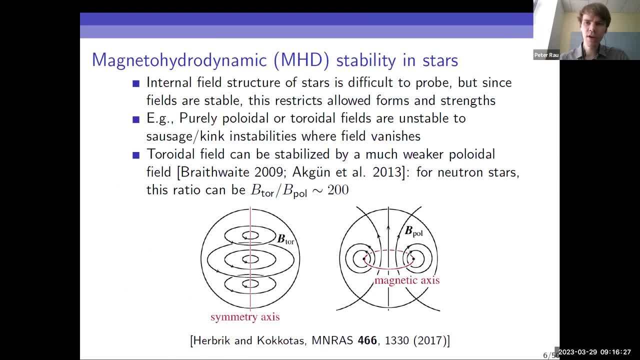 So it's still an inactive area of research. So one of the things you want to have to consider if you're going to look at, you know, MHD instabilities triggering These emission events is the overall, you know, stability of a magnetic field in a neutron star. 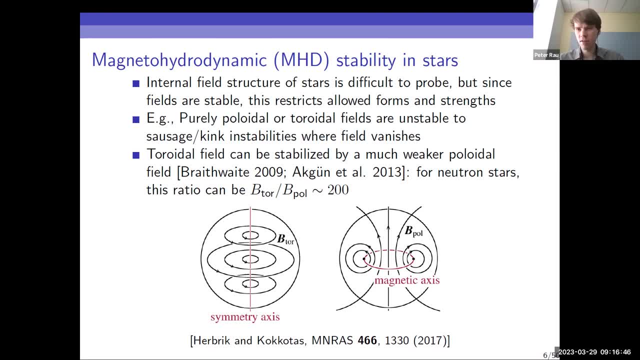 So the internal magnetic field of any star is difficult to probe. You can't just stick a gauss meter inside the star and measure the field. But we can observe the field which is emerging from the star and we can use different theoretical tools to limit the allowed forms and strengths of the field. 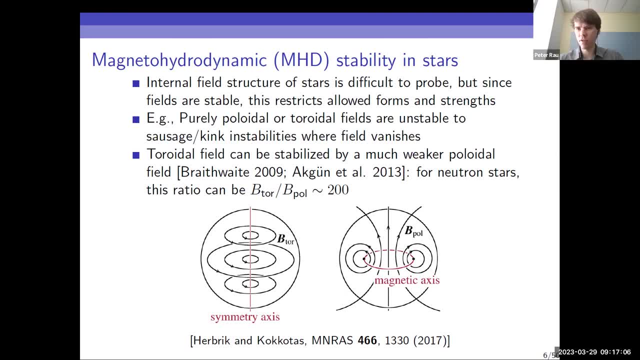 But we can observe the field which is emerging from the star and we can use different theoretical tools to limit the allowed forms and strengths of the field, Because the field is stable over long timescales. It is evolving, but it's evolving very slowly and in a controlled manner. 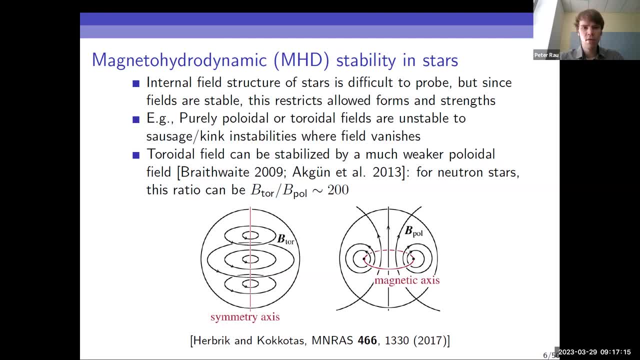 It's not just becoming unstable. So, for instance, we know that a purely poloidal field- so that would be like a magnetic dipole, like that shown in the lower right here- is unstable, And similarly a purely toroidal field like that on the lower left, is also unstable. 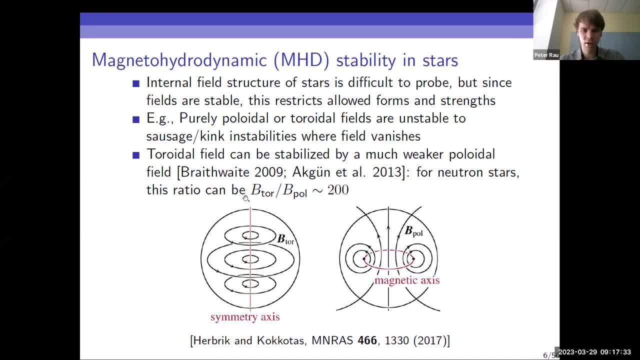 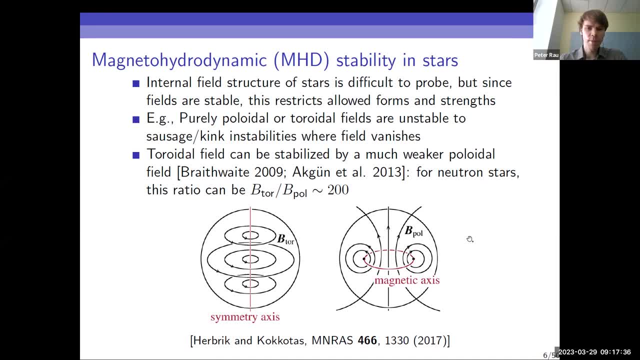 Along the axes where the field vanishes. But if you superimpose these fields you can stabilize them to each other because you now no longer have a vanishing field along this axis or along this axis. And for a neutron star, the ratio of the toroidal to the poloidal field can be, I guess, 200, while retaining, while being stable. 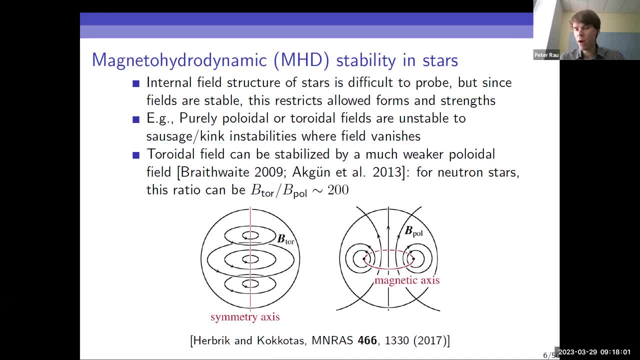 So the idea is that there's a lot of things we may not know about the magnetic field of a neutron star, because you have a much stronger toroidal field which we can't really measure that well inside the star, because it's only the poloidal component which is emerging. 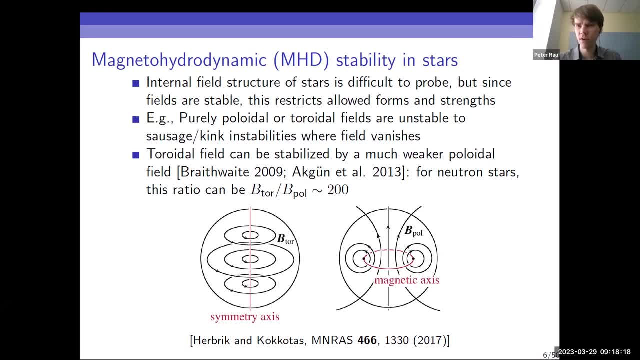 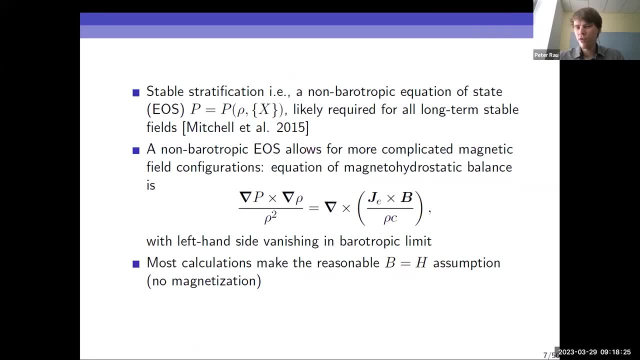 from the star and you know which is responsible for the surface field that we can sort of indirectly measure. So the reason for that high ratio in a neutron star is the equation of state and the effect of stable stratification. So basically that means that you have a non-barotropic 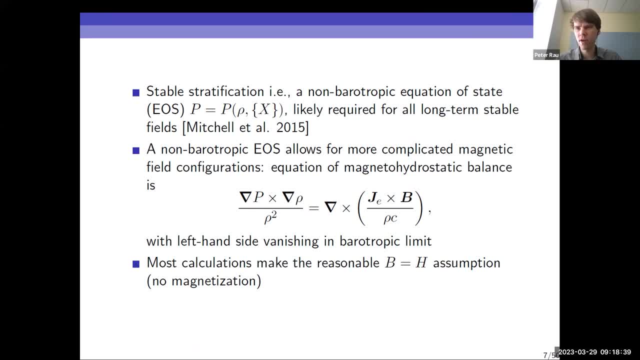 equation of state or the pressure is not just a function of the energy or mass density. non-relativistically, It's a function of different chemical species fractions, like the proton fraction and a neutron star. So that would be the most important of these chemical species fractions. 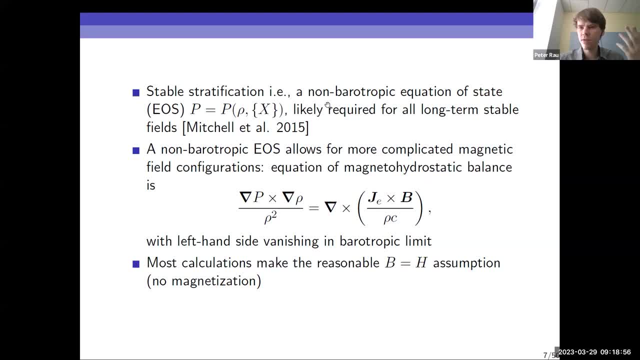 And it's likely required that you have such a stable stratification for any very stable stratification, So that would be the most important of these chemical species fractions. long-term stable field in a neutron star. A non-barotropic equation of state- also allows for. 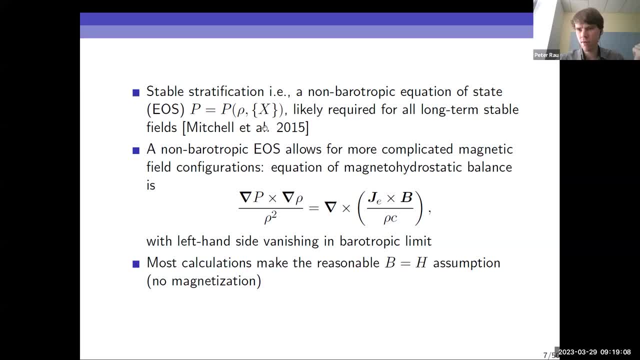 more complicated field configurations. So if you don't have, if you just have, a barotropic equation of state, the equation for MHD balance takes this form. And so if this side was zero, as it is in a barotropic EOS, then you're restricted to forms of the magnetic field which satisfy J, cross B over. 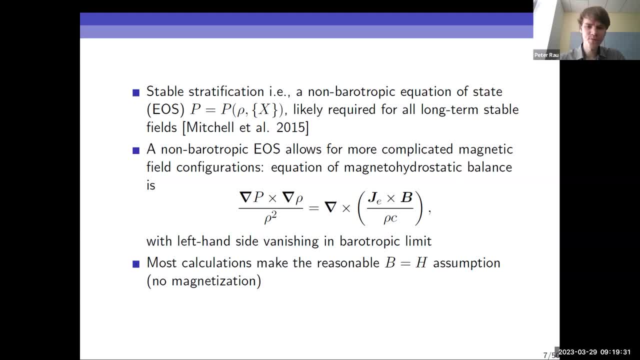 rho C. So the answer to that is that the MHD is the grading of a scalar which is quite restrictive, And so these are some more general results from MHD stability. but one thing that is commonly assumed, and especially in lower magnetic field stars, is that the B and the H fields are the same, That there's no magnetization going on. 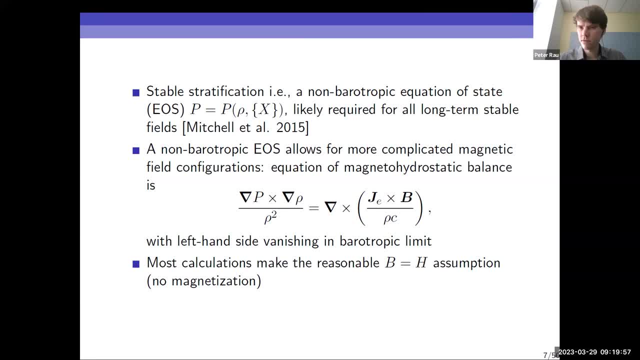 It is. if it's not relevant at for a while now is: is that always going to be true in magnetars Or is there something which is changing that here, Because we do have very strong fields, And what does change this a bit? 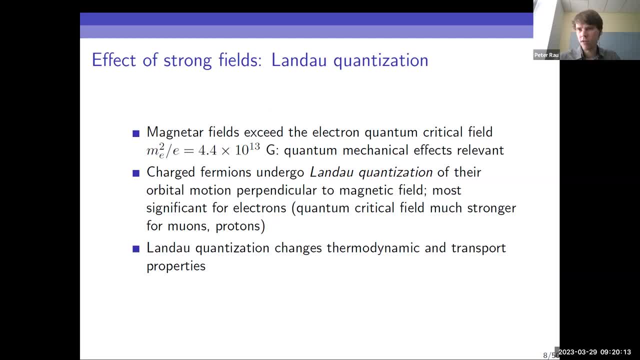 is Landau quantization, So magnetar fields sort of reach and exceed the quantum critical field for the electron, So that's around 4.4 times 10 to the third of the chaos. And so once you reach that, there's some quantum mechanical effects which become of importance And in particular, 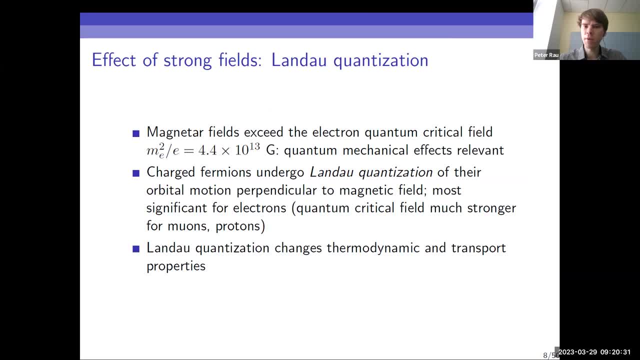 the orbital motion of electrons perpendicular to the magnetic field becomes quantized Again. this is Landau quantization, quantization of cyclotron orbits. This happens for all charged fermions at some magnetic field, but it's really most important for electrons because this critical 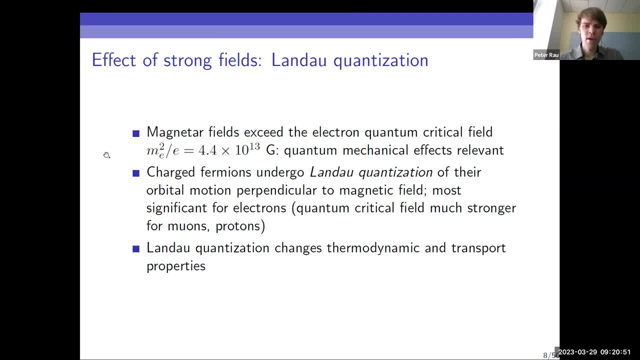 field scales as the mass of the particle squared. So you have to get 10 to the 17 gauss for muons and like 10 to the 20 or so for protons. So it's not really as relevant for them. And Landau quantization is known to change thermodynamic and transport properties in some. 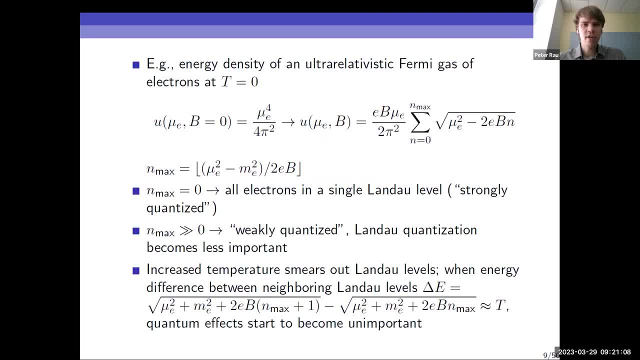 quite dramatic manners. So, for example, if we look at the energy density of a ultra-eligivistic Fermi gas of electrons at, let's say, zero temperature, in the zero field case it just scales as the chemical potential to the fourth. If you add the field in, you now have this sum. 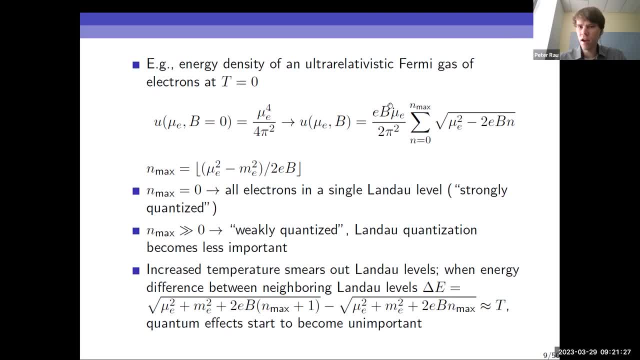 over Landau levels And these field terms appearing in the energy density. So this sum starts from n equals zero, and goes up to some maximum occupied Landau level, which is determined by the Fermi momentum squared over 2 e b. So if you have a very strongly quantizing field, such that n max is zero, then you only have 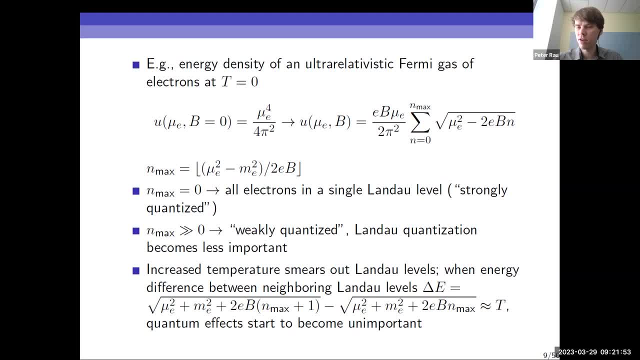 one Landau level being occupied. So it's known as the strongly quantized state, And the energy density here has the same dependence on the chemical potential as a 1d electron. Yeah, so it's. sometimes the system is known as one dimensional. at this point The electrons can just move along the field. but 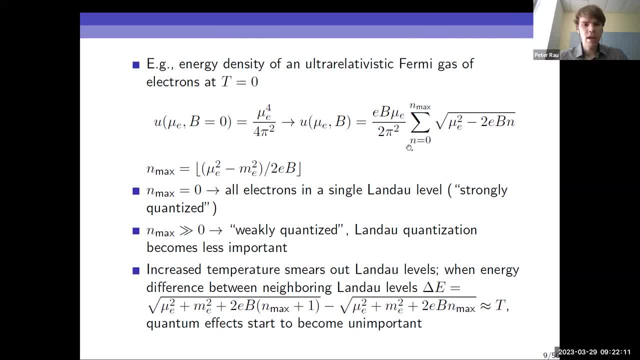 they're really restricted from moving perpendicular to it. If you have n max being larger than, let's say, like a few, then you're said to be in the weakly quantized regime, Landau quantization is. you still get the certain effects from it, but it's not as important as it is in the 1d regime. 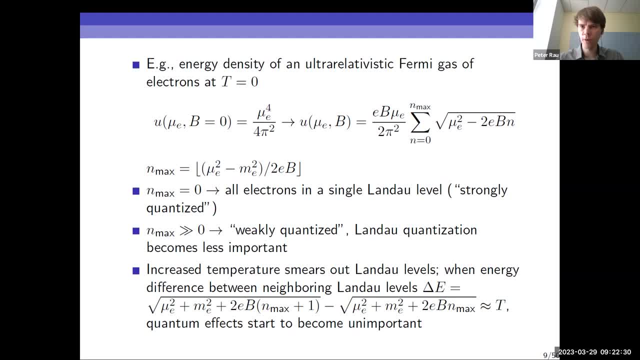 And these effects start to become blurred out by temperature. So when the temperature of a system is about the same as the spacing between the highest occupied Landau levels, then these effects become not entirely irrelevant, but they start to become less noticeable. So what effects does this have on? 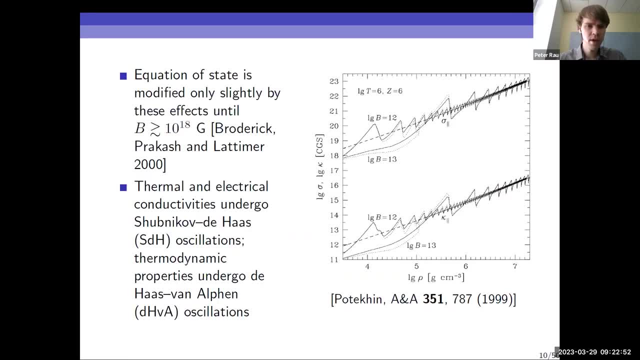 different properties relevant for neutron stars. The equation of state is very minimally modified By Landau quantization until you get to fields of order 10 to the 18 ghosts or so. but we know that those fields cannot exist at a global scale in a neutron star because it would 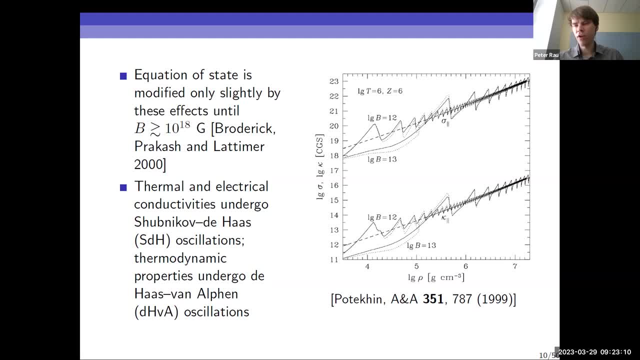 make the star unstable. The gravitational binding energy would be overpowered by the magnetic field, So that is of sort of lesser importance, except maybe in the outermost layers of the star, So in the outer crust, it can have some effect. Now we also know that. 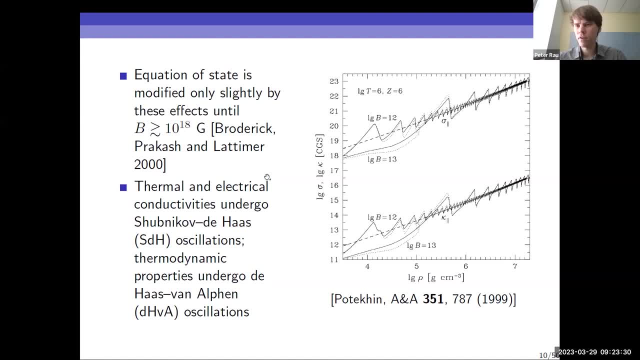 there are these oscillatory effects, which occur in different transport and thermodynamic properties. So, for instance, the thermal and electrical conductivities undergo what are known as Shubhnikov-DeHaas oscillations, And so I've illustrated some of these to the left here. 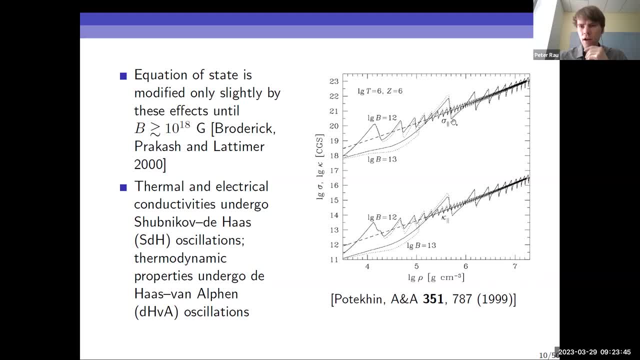 or sorry, to the right rather. So we have the conductivity, electrical and thermal parallel to the magnetic field, plotted as a function of density. So this is a typical like outer crust, very outer crust. And then we have the oscillatory effects which occur in different transport and thermodynamic properties. So, for instance, the thermal and electrical conductivities undergo what are known as Shubhnikov-DeHaas oscillations, And so I've illustrated some of these oscillatory effects which occur in different transport and thermodynamic properties. 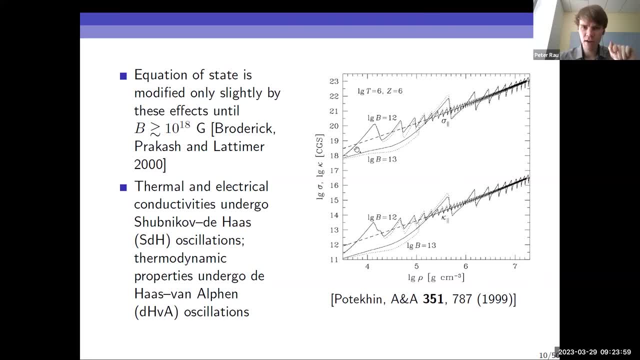 So for instance, the thermal and electrical conductivities undergo what are known as crust densities for fixed temperature and then different field strengths. So if we ignore the Landau quantization entirely, we get the dashed lines here. If we use a field which is 10 to the 12 Gauss, 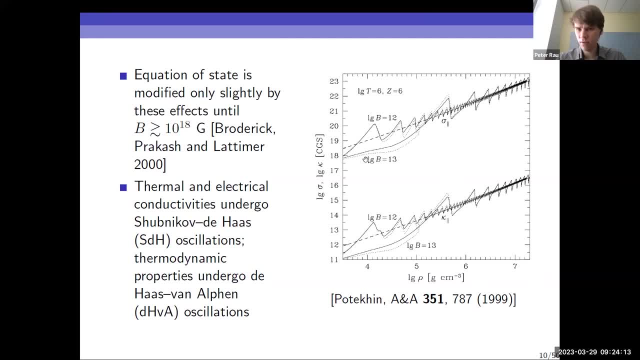 you get this first solid line, And if you increase that field by a factor of 10, you get the second solid line. And you see that as you increase the field, the amplitude of the oscillations becomes larger, but the sort of spacing between them becomes larger as well. 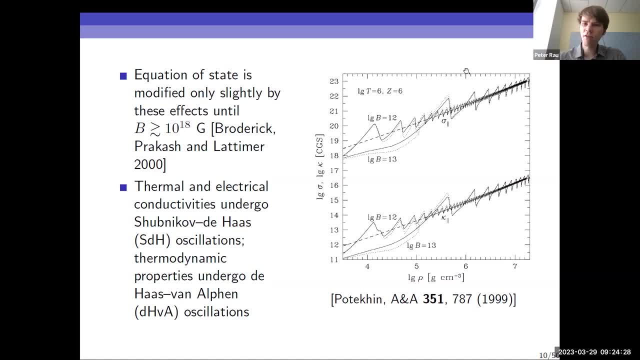 because you know there are fewer Landau levels being occupied And these oscillations have to do with where you are alternately filling up or emptying new Landau levels, depending on which way you're approaching it. But the thermodynamic properties also undergo oscillations And these are related but undergo. 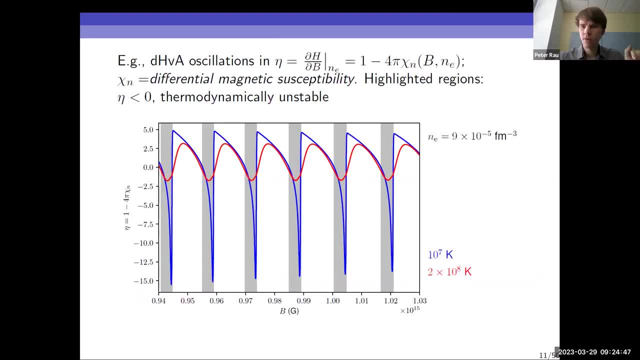 under a different name, DeHaas-Span-Alphain oscillations, And one quantity of particular importance for the rest of this talk, which undergoes these oscillations, is what's known as the differential magnetic susceptibility. So you can expect valence, or we can, you know, write this eta quantity. 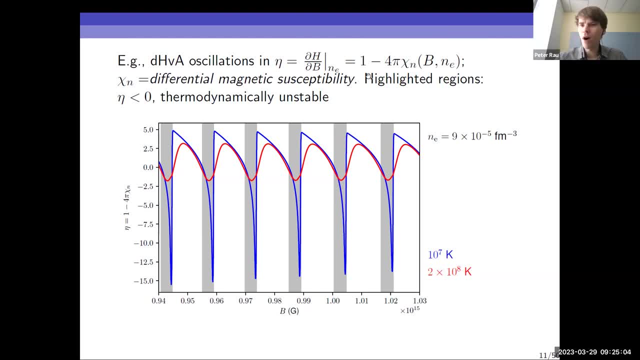 a partial derivative of H respects to B And what's you know what? What is different from just one here is this Chi n quantity, And so what I've plotted on this figure is this: eta quantity is a function of a field for fixed density and at different temperatures. 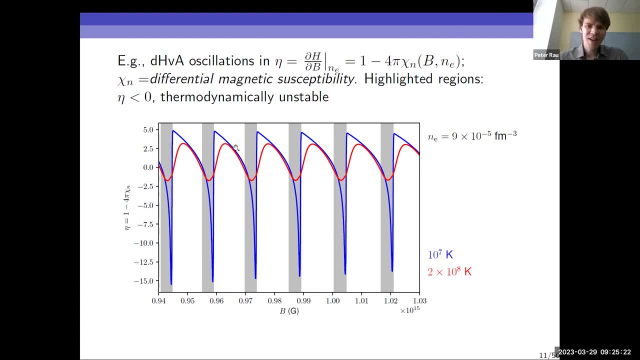 So you see, the temperatures are suppressing the oscillations, but still, like this eta quantity by four pi can be of you know order unity. maybe bigger than that can be like 10 or so potentially at um, depending on the exact parameters, um, but parts of this are sort of not they're relevant. 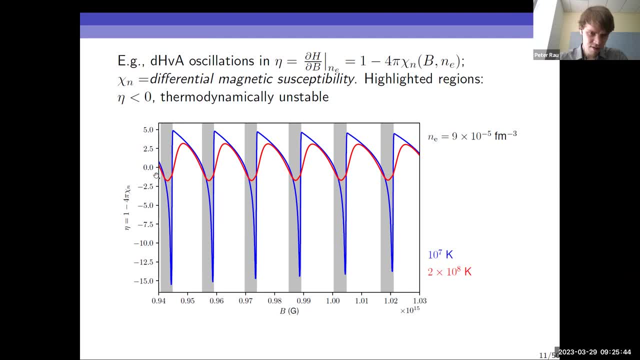 but they're of sort of maybe more academic interest, because these dips here are, um, thermodynamically unstable. so if eta is negative, there is a thermodynamic instability which has to be resolved somehow, and i'll get back to the resolution of that a bit later, but still you 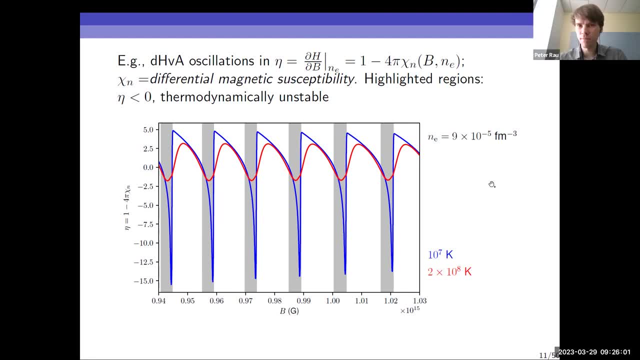 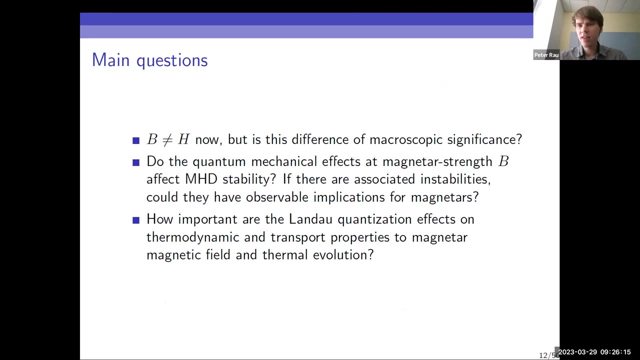 have these large oscillations which are um, thermodynamically stable, um, which are the regions where this is positive, um, and you know, larger than one, so um, that is sort of like the sort of end of the introductory part. um, we see that, you know, b is not equal to h, but is that? 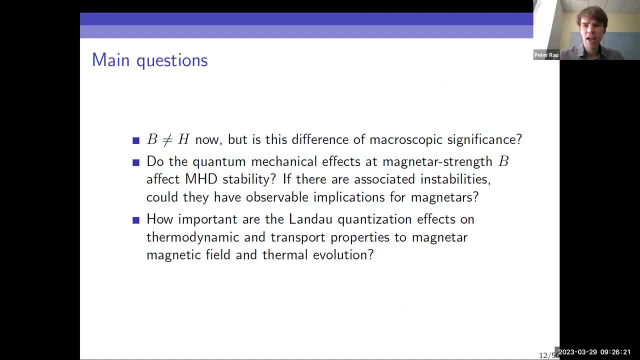 difference of macroscopic significance, um in particular, can these effects model modify mhd stability of a magnetar and could they have observational implications? if so, and finally, what is the importance of lando quantization effects on thermodynamic and transport properties to the evolution of the magnetic field and temperature of a strongly 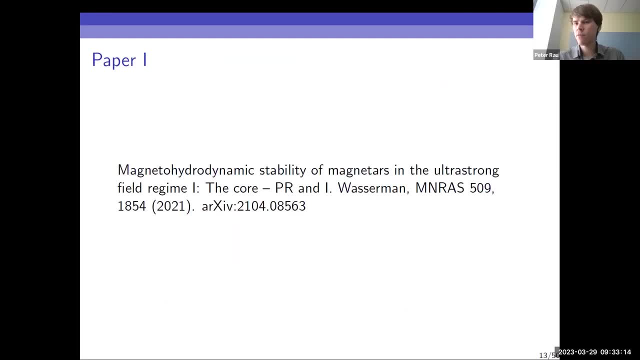 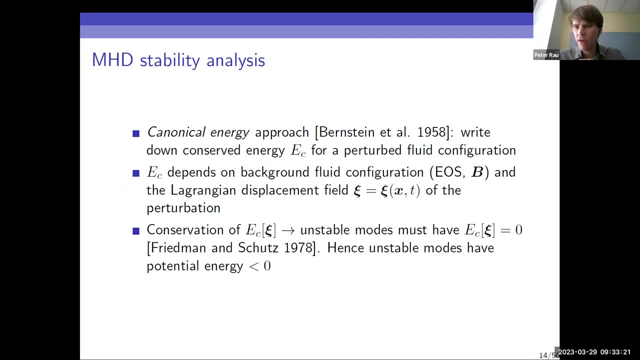 magnetized neutron star. okay, so again i'll first be talking about what happens in the core of the neutron star. so, um, we try to do a stability analysis in the core of the neutron star and the core, and there you can make use of what's known as the canonical energy approach. 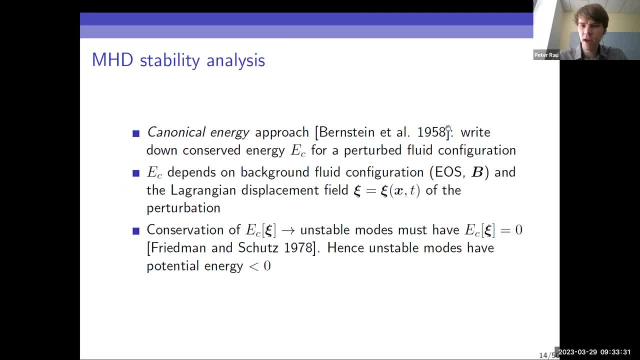 this was developed interestingly by people working on a feasibility of a nuclear fusion reactor and the idea is you write down a conserved canonical energy for a particular perturbed fluid configuration. this quantity, e sub c, depends on the background fluid configuration, the equation of state in the field and also the displacement field which tells each fluid element how to move. 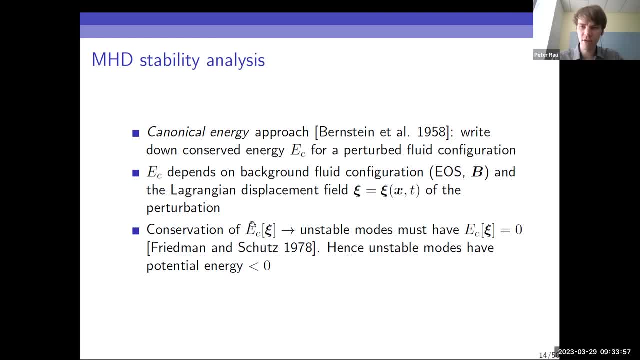 when you perturb the fluid, you can show that this quantity is conserved, and so if you have an unstable mode, it has to have e sub c being zero, because otherwise it would grow exponentially, and so that means that we can look for modes which have a negative potential energy contribution for 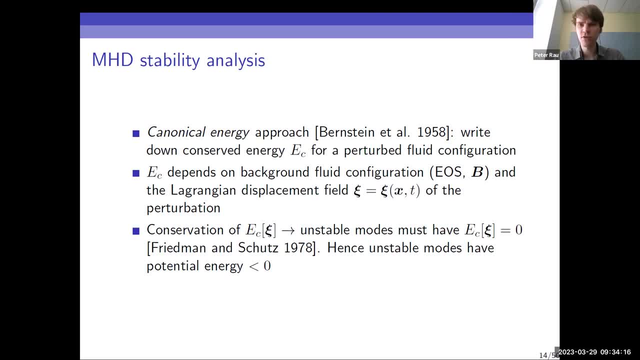 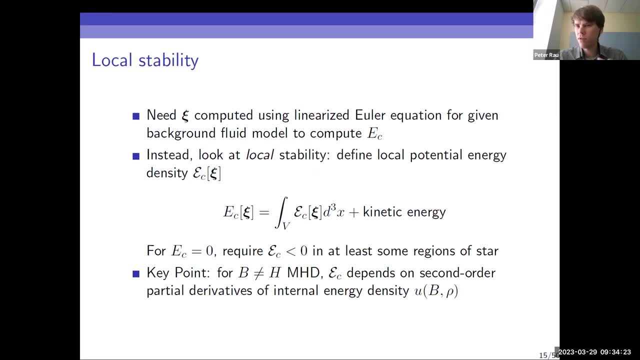 we're going to find one which is unstable because the kinetic energy contribution will always be positive. but this tends to be quite a complicated procedure. you need to use a linearized Euler equations and solve for the displacement fields in the same manner you would for solving oscillation modes for, for example, like a star. but now we have all these additional. 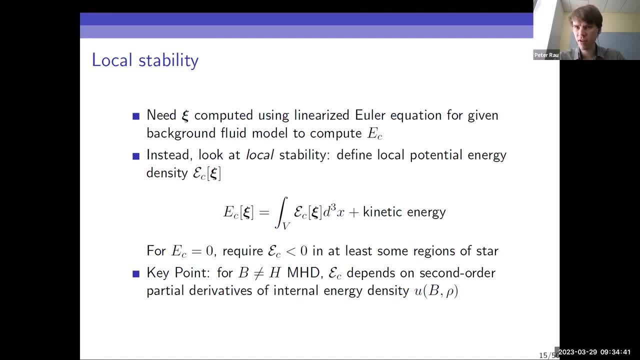 complications put on top of that, like the magnetic field and the land of quantization effects. so instead we looked at local stability. so we defined a potential energy density which, when you integrate it over and then add the kinetic energy, you get the total canonical energy. and if you want this to be, you know we're looking for regions where you could have potential. 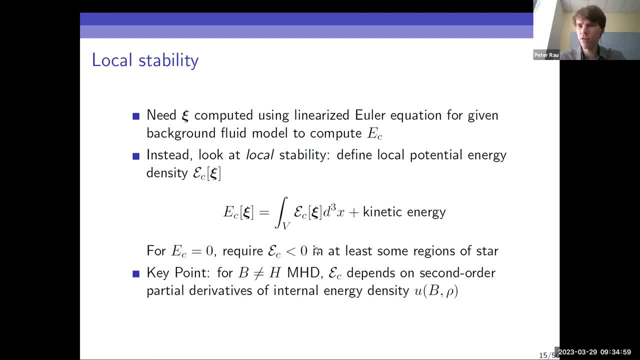 instability. this needs to be zero, so this energy density would have to be negative somewhere. and the key point for us is that this quantity depends on derivatives of the internal energy density of the system, which depends on the field and, like the mass density and the field contributions, will give rise to things like the magnetization. 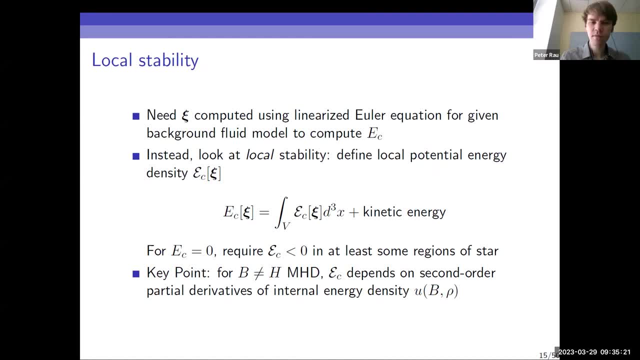 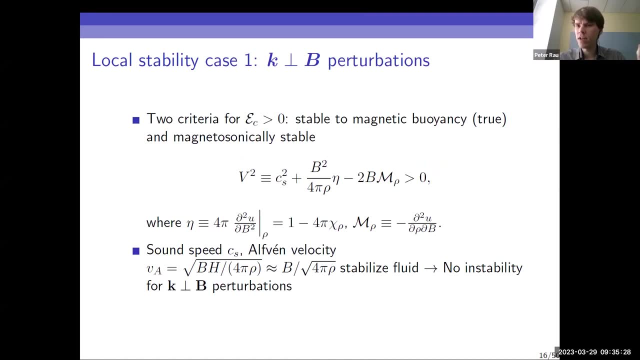 and this differential magnetic susceptibility. so it turns out to be easiest to examine these different stability cases in terms of the orientation of the wave, vector of the perturbation and the magnetic field. and so if we look at the case where these are perpendicular, there are different terms which appear in this quantity script, you see, and if we want to look at 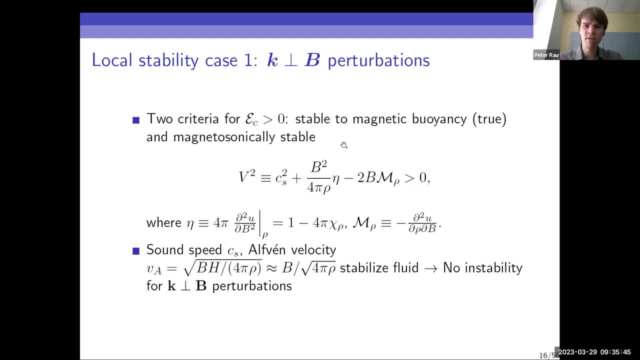 want to ensure stability, rather we have to guarantee this is positive. and one of these contributions has to do with the something called magnetic buoyancy. i won't really go into that in too much detail, but the other contribution has to do with this sort of magnetosonic speed squared and this needs. 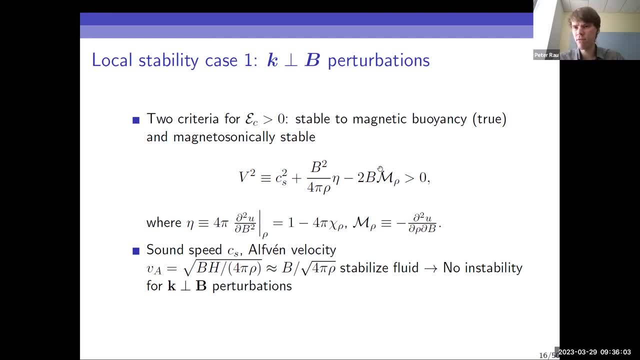 to be positive. so this is the velocity of magnetosonic waves, which are one type of mhd mode, and this will generally always be zero in a neutron star core, because the sound speed is huge there, um, and so that this term will over power these other two terms. so you can see where the contributions from the lando quantization come. 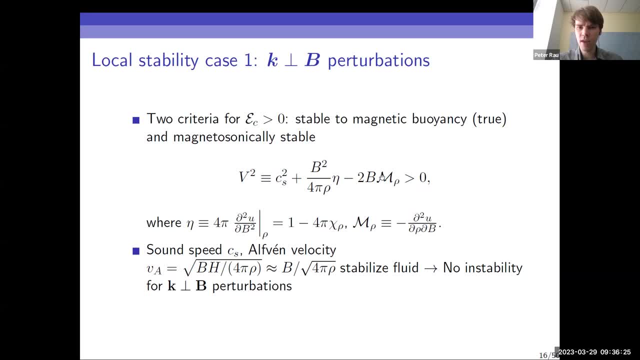 in here. they come in from eta and from this um m sub rho, which is the mixed partial derivative term having to do with the magnetization. so it's the derivative of magnetization with respect to mass density. um, it turns out that because of the stabilizing effect of the sound speed there is 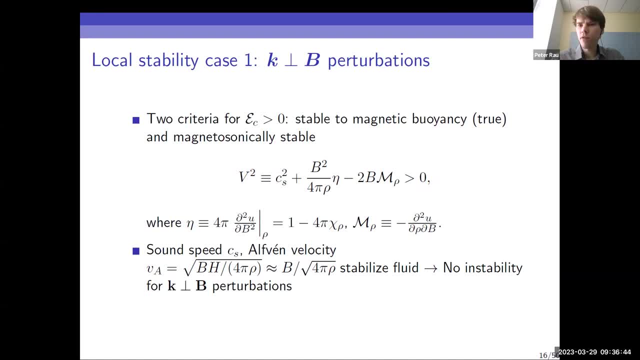 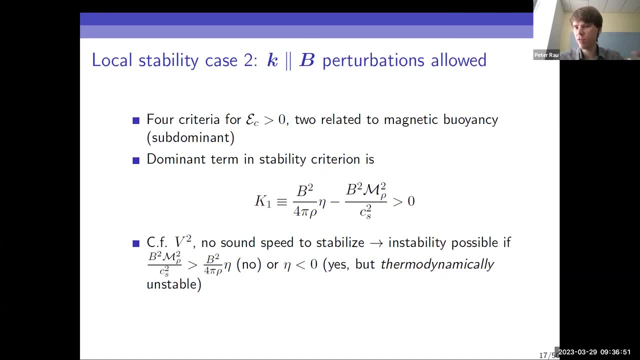 no instability possible for this type of perturbation. so if we consider the second type of perturbation now, we have k per per. so if we consider the second type of perturbation now, we have k per per, or sorry, k parallel to b and that is um. these oscillations are more like alphane waves. the 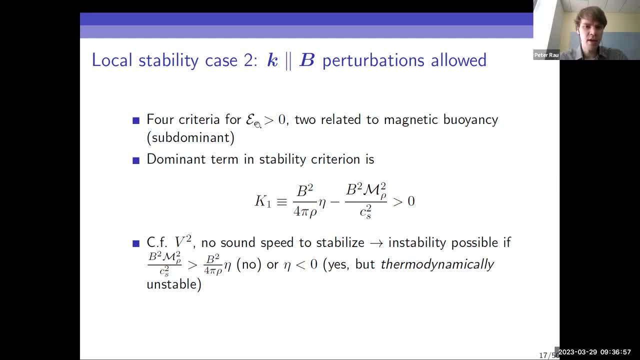 oscillation travels along the field um. the uh script ec is more complicated. here there are now four different terms you have to worry about: um, one of which um or two of which depend on magnetic buoyancy, but those are subdominant and the dominant term is- i've called it uh k sub one. 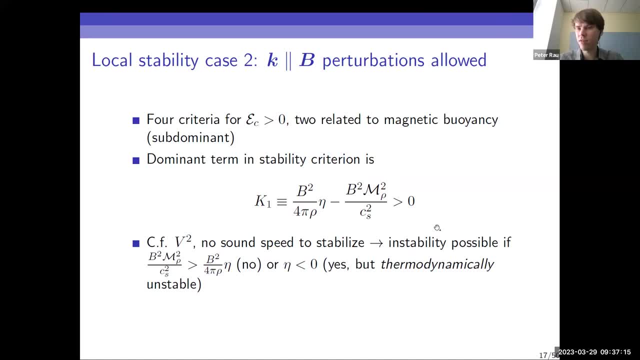 and it is given by this expression here. so this could be negative, because you don't have this sound speed squared stabilizing you, um, but it can only be negative if this term is larger in magnitude than this one, which turns out to not really ever be true, and then, or if this eta could be negative. 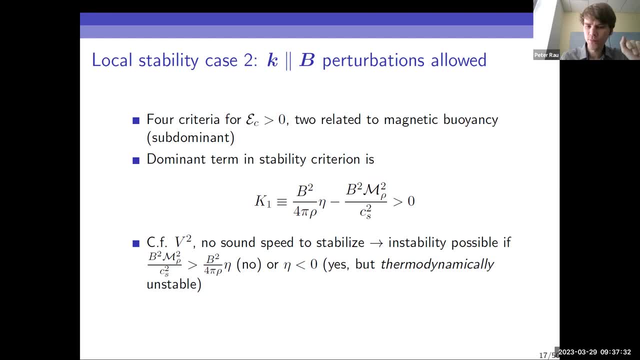 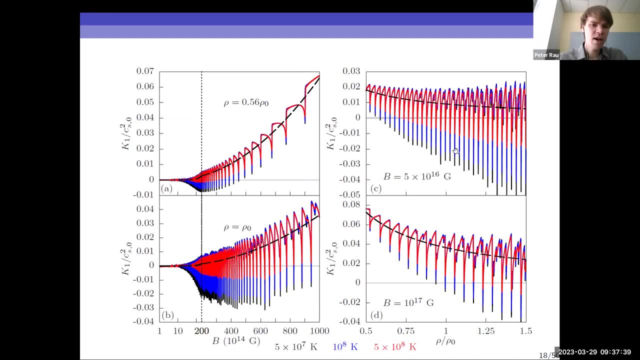 which it can be. but that sort of implies thermodynamic instability as well. so if we just plot this quantity, so where could this be potentially unstable? and we see, um uh, that it can be unstable in you know quite a range of uh. we have densities and fields here and i've also 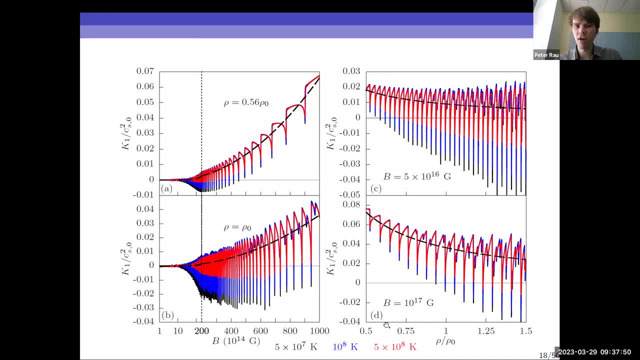 shown this a different temperature. so again, finite temperatures suppress these oscillations um. but interestingly it turns out that this is not really relevant in the most strongly quantized um regions. so for example, if we look at this lower density region, this is about half the nuclear saturation density um. we see that 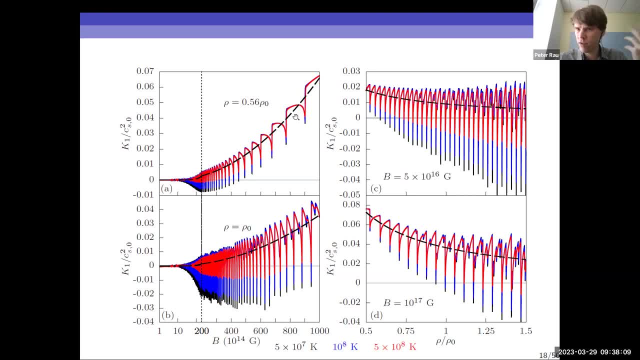 once the field gets sufficiently strong, once a small number of lander levels is occupied, um, you never actually go below um this, you know zero line, and then at that point you know you would be purely stable up here, um. and similarly for lower densities and higher. you know fixed fields. here you are never unstable. but once you get to higher, 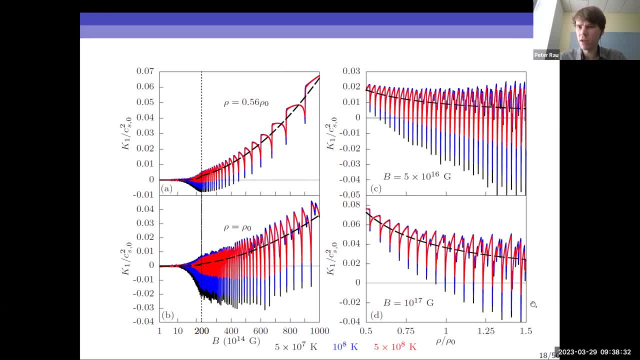 densities, and it's still the same field. um you can be, uh, unstable again. um i'll point out that um the sort of regularity of these oscillations starts to shift it once you um reach this density where muons come in. so that's what these sort of sub-dominant oscillations are. 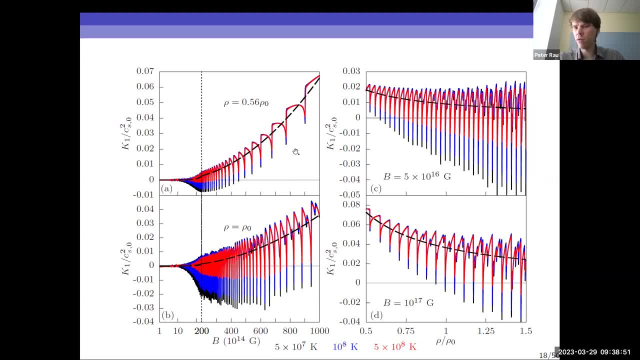 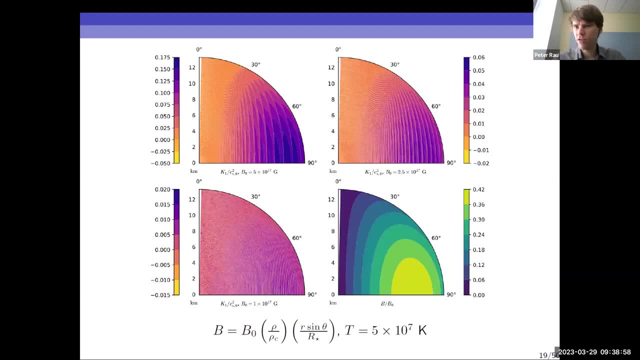 you can see here and here and here to some extent, but you don't see in the upper left because there are no muons at that density. yeah, um, this is just showing what this looks like inside a cross section of a neutron star. so we've assumed a purely toroidal magnetic field with its maximum. 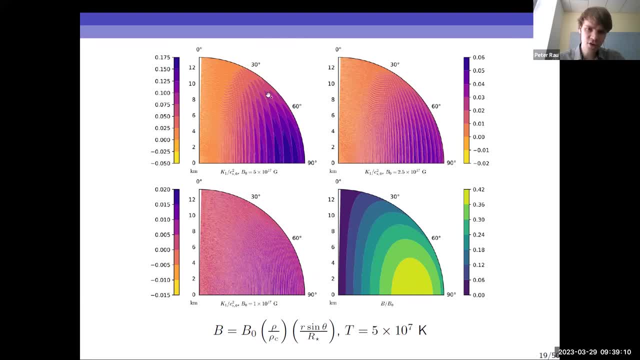 in this outer region, here, um, and the potentially unstable regions form sort of like shells um in the star. so we're looking at sort of the regions where this is um these colors are like in the yellow or orangey- where things become negative um, where you could potentially have this instability, um active, um, and the idea is that 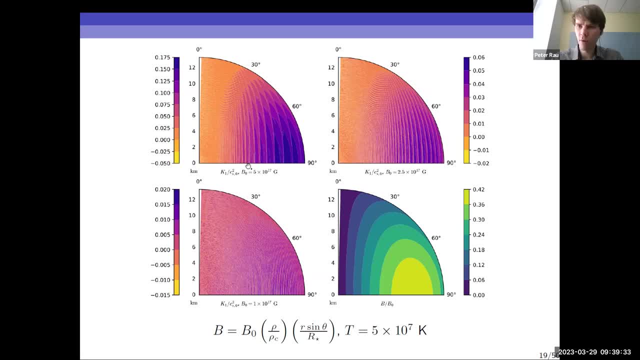 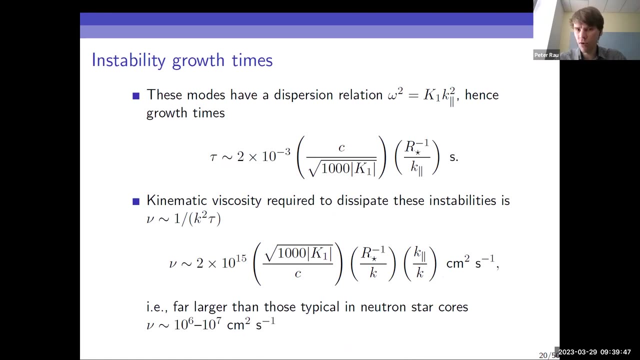 as you d, as you decrease the field, you have more of these regions forming, but you're getting these sort of shell-like regions. of course it's depends on the field structure and the density gradient. this instability, if it is active, grows very quickly. um growth times are. 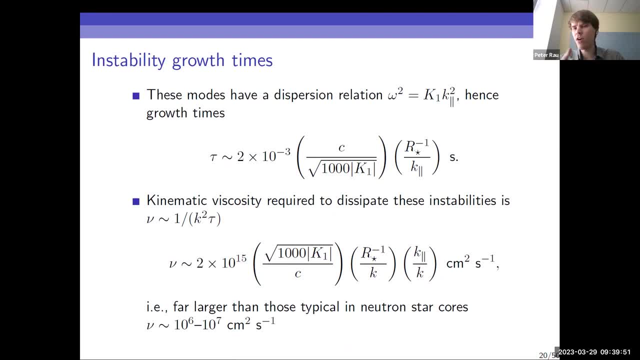 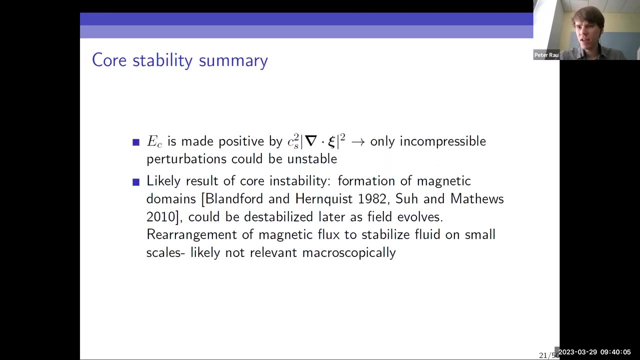 basically a constant um, because this instability is not active and it's below the negative order uh millisecond. so I'm just going to try to kind of avoid that further with just some uh action and more of the. the International theory of space and space and time. 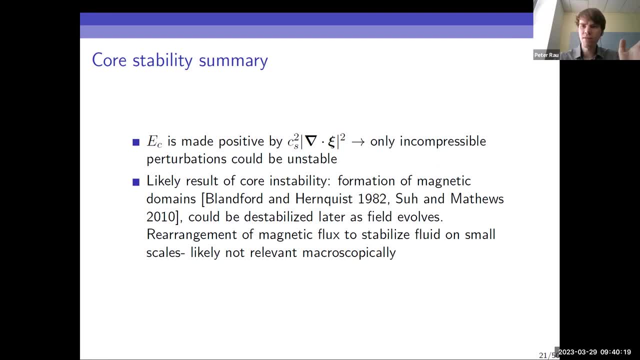 were once stable now become unstable. but the effect of that would most likely be: um, you have maybe a very brief period of instability, growth until of growth of the instability, until you rearrange magnetic fields to um, essentially cause the domains to form again, but at different locations, and so it's not really of any macroscopic relevance, because it's- i mean it's- 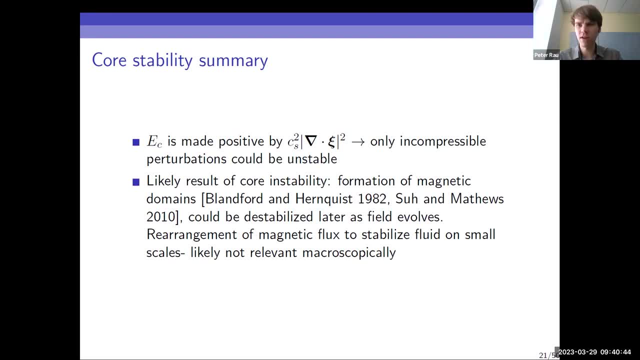 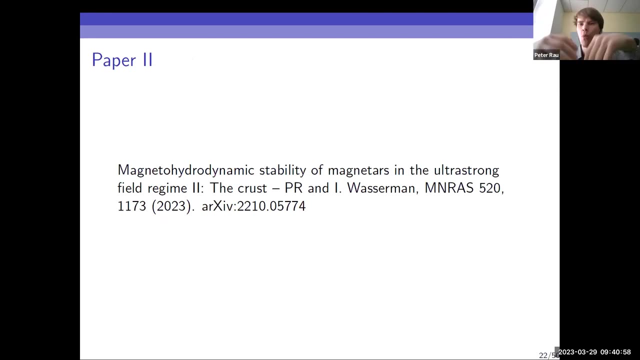 so deep in the star anyway, that the effects would just be quite, um, excuse me, uh, minor, um, uh. so maybe what happens, something happens a bit different in the crust, so i'll look at the crust now. um, so again, the crust is. you know where the emission is coming from. um, so maybe this is of 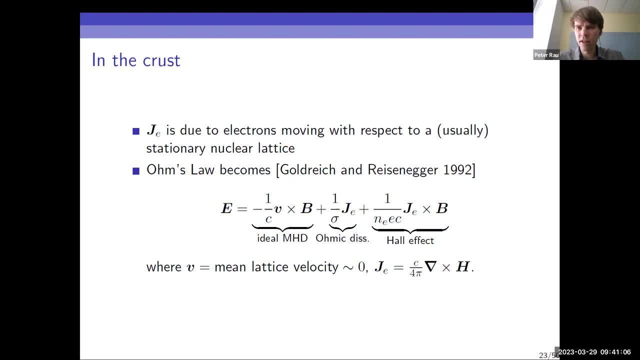 more relevance. um, and the physics in the crust is slightly different. so in the core, all of the charged species move together and the physics in the crust is slightly different. so in the core, all of the charged species move together. um, it's a plasma, but the crust is a solid. you have. 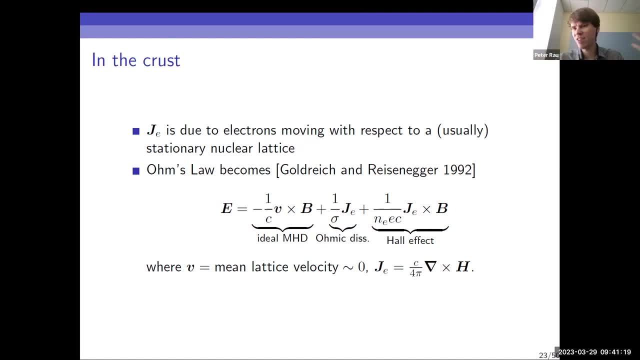 electrons moving with respect to a stationary nuclear lattice and so it's similar to a metal. and because of this difference you have to modify the expression for ohm's law, so you have to add additional terms into the electric field. so an ideal mhd like we used in the core, you only have 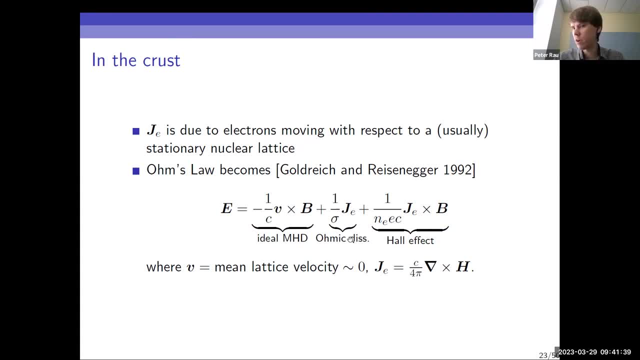 this first term in the electric field. of course you could have omic dissipation as well. um, i guess by ideal we mean we ignore this usually, but it's in there technically. but because the conductivity is much higher in the core than in the crust, it's more relevant in the crust and then 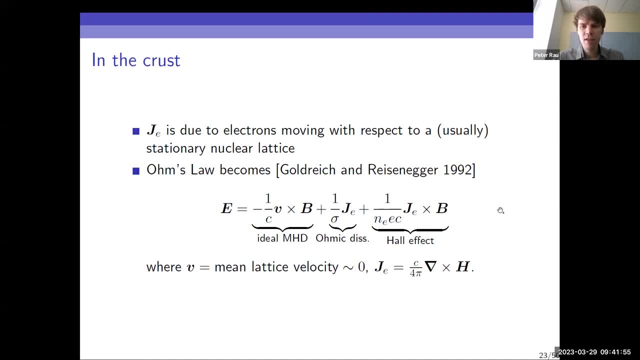 finally, we have the hall effect term um, and so one thing to note is that if the velocity of the nuclear lattice is about zero- we're assuming it's stationary- then you ignore the ideal mhd term, and for you know our purposes. what's really interesting is that j is the curl of the 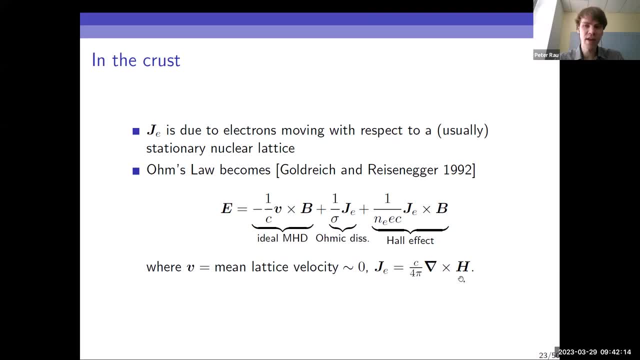 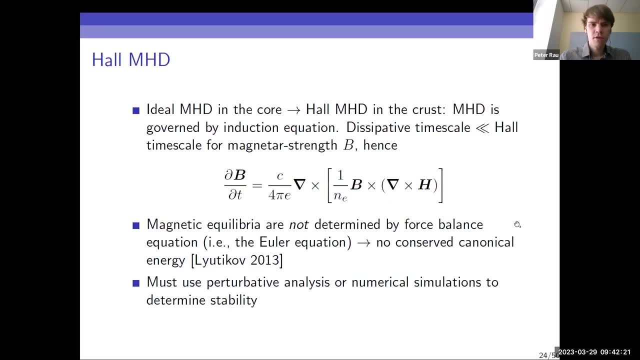 h and because of that you have magnetization effects due to landau quantization which come in through this term and, of course, also through this term here. so, effectively, what you've done is gone from a regime where ideal mhd works in the core to one where hall mhd works. so that's. 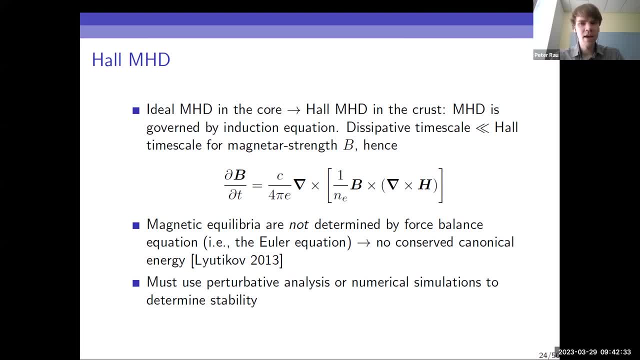 what we call this type of um, mhd, um and the dynamics of the field are governed by, not like a force balance equation, but by the magnetic induction equation or faraday's law, um, if you can assume that the time scale for the hall term is much shorter than 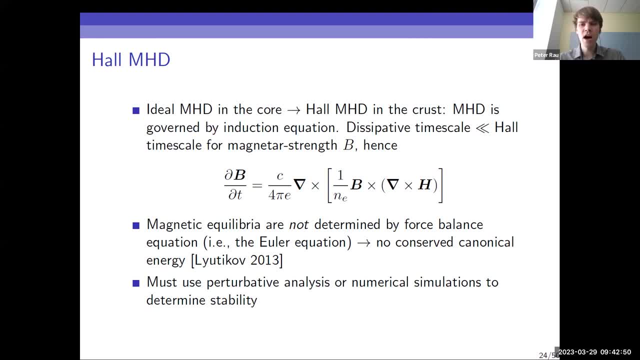 the time scale of omic dissipation, which is generally true, um, and is definitely true for magnetar strength fields, then the equation governing the evolution is this one here. so, in equilibrium, the field is not evolving, this term is zero and you are left um with an expression. 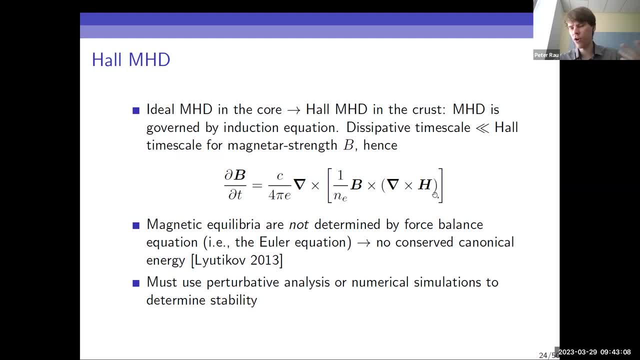 for an equilibrium field, that this term in the square brackets is the gradient of some scalar. but because of this um you can't derive a conserved canonical energy. um, in hall mhd you have to do something different to study stability. so what we do is, uh, use perturbation analysis. 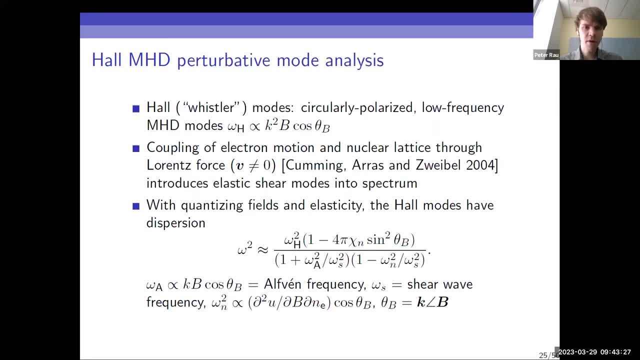 and so we have new modes which enter the oscillation spectrum. these are known as hall or whistler modes. they're circularly polarized, have low frequencies and notably their frequency scales as the wave number squared, as opposed to just the wave number um, as it does in the ideal mhd case in the alpha and magnetosonic. 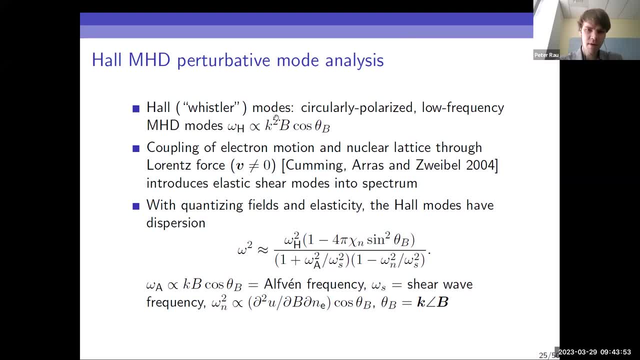 um, there are different effects. we can, you know, supplement um this with. so this is the dispersion for hall modes, when you ignore um coupling to the crust and things like random quantization. so, um, one thing which is a sort of importance for magnetaries especially, is um, 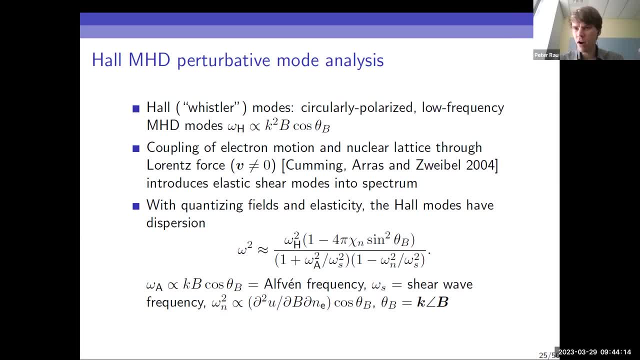 that the magnetic stresses are very strong, and so the force is acting on the crust due to the, you know, the lawrence force are strong as well, and so, um, we can't consider the solid lattice of the crust to be, you know, perfectly rigid. you have to account for, um, its elastic response, and you get. 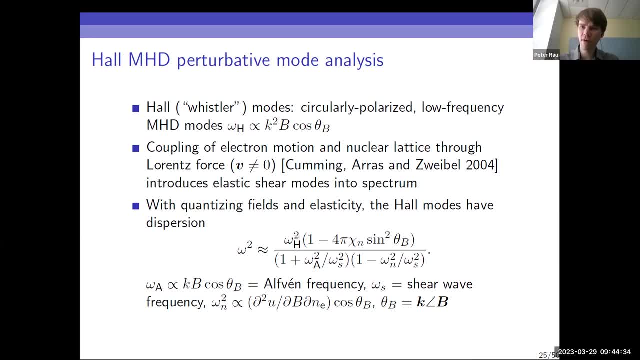 elastic shear modes. from that they add to the spectrum and they also modify the other modes. so if you include elasticity and quantizing fields, the hall modes have an approximately lower pump progressive bond. so in our case mth is a sort of higher typical motion than the. 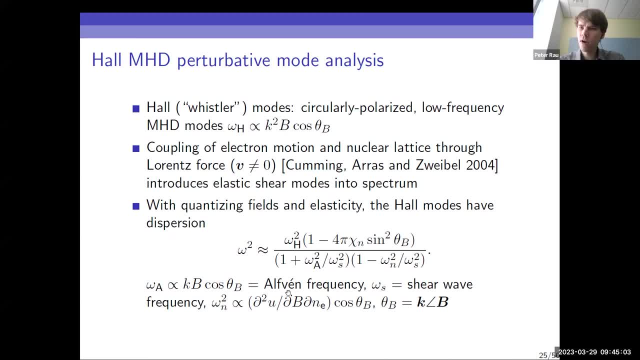 real mode which might be in your project, but if you're looking at a higher typical mode and you do the same kind of Brahmsian två moves like what's being shown as a continuous translation according to convective mode x to f i in the unquote i'm guessing those things are quite wellganides. 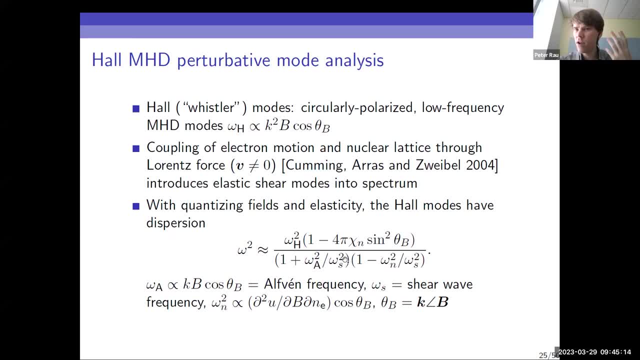 essentially zero. but if the field is quite strong, um, and is, you know, be comparable in strength to the shear modulus, um, you know, with some other factors in there, um, then this can be significant and can suppress, uh or lower the frequency of these home modes. now, is there a possible? 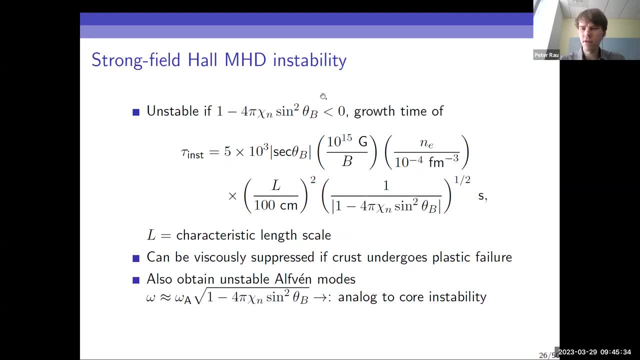 instability here. technically, yes again, um, if this term on the numerator is negative. but the growth time is much slower than it is for the alpha type modes because, um, the hall modes have, uh, lower frequency and so it's about a million times slower growing than the unstable alpha type modes, which, 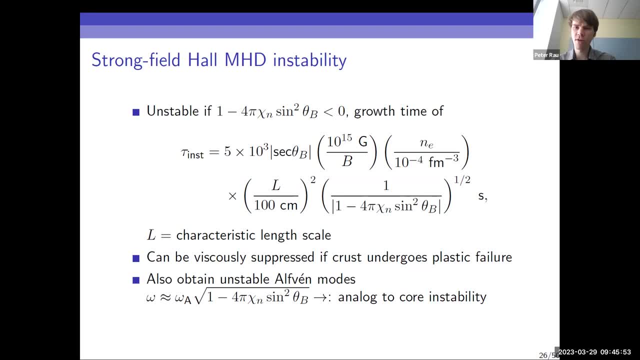 still do exist in this spectrum. it's like the hall modes are an additional mode on top of them, that appears, and i'll point out that all these sort of instabilities could be suppressed by um the crust undergoing plastic failure because, um, i haven't really mentioned this- the the crust. 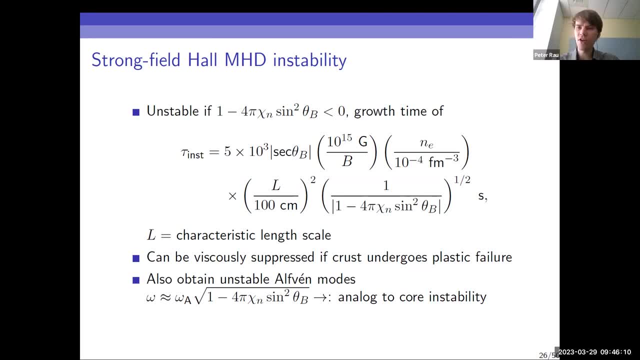 um. it's not really expected to sort of crack brittly, but it undergoes a sort of a more gradual failure in which you replace essentially a sheer modulus with a sheer modulus plus some like frequency dependent um term which incorporates an effective viscosity um once you exceed a critical. 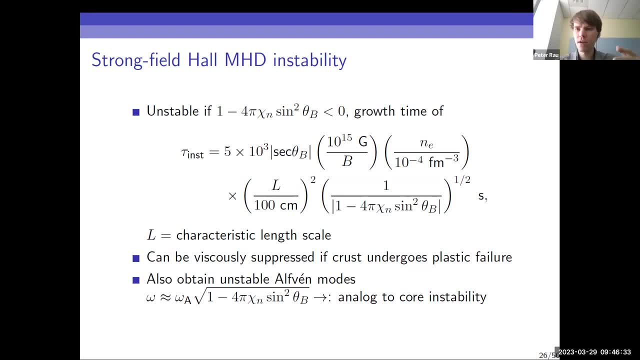 uh, magnetic, uh stress acting on the um lattice and if that is of a sufficient strength they can suppress this instability entirely. But there's still a lot of details about the plastic nature of magnetar and neutron star crust which are not fully understood. but it's a very interesting field at all. 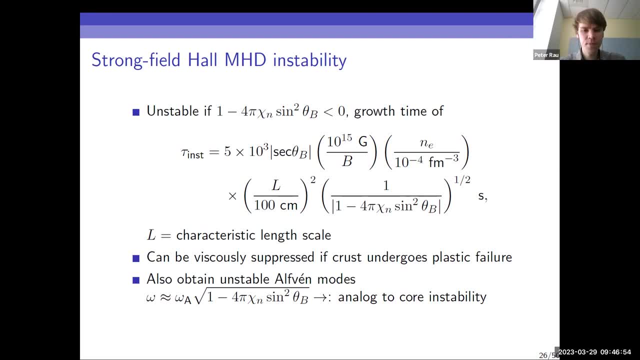 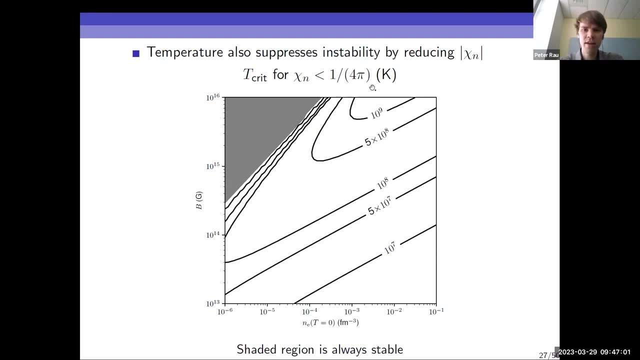 So I'll leave my discussion at that for now. Additionally, temperatures suppress this, of course. So if we look at the critical temperature for chi sub n to be less than whatever four pi, ie for the sensibility to be not possible. 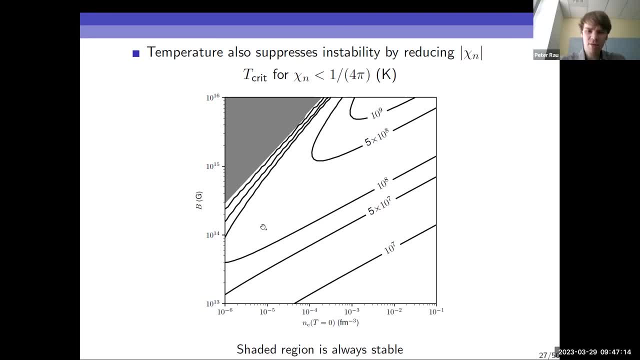 we see that again, it's more at higher fields and lower densities. You'd expect you to be unstable, because that's where these oscillations are biggest, but it turns out that, again, the sort of strongly quantizing regime- you're always stable. 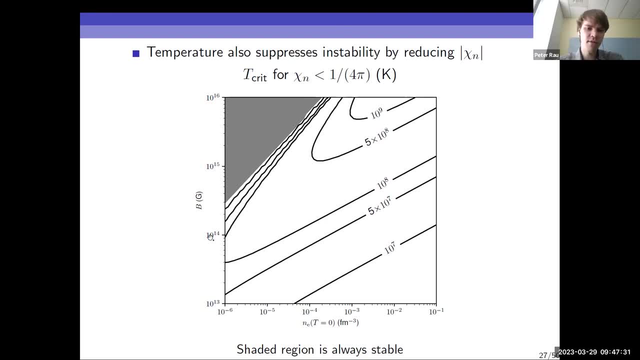 and it's more the intermediate regime. which things are interesting. A fixed magnetic field, let's say 10 to the 14 Gauss and increase the density slowly. you start off being stable above 10 to the 8th Gauss or 10 to the 8th Kelvin. here, 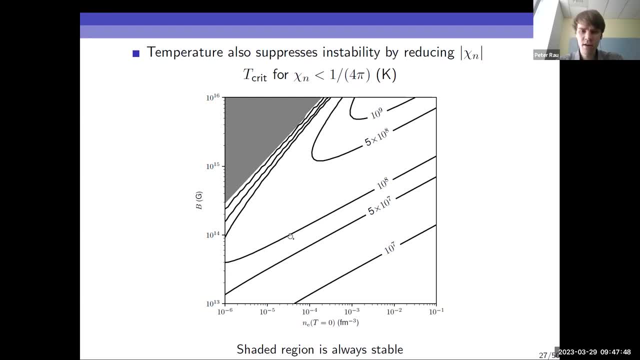 Once you reach this curve, you are now only stable below 10 to the 8 Kelvin, now only stable below 10 to the or 5 times 10 to the 7 Kelvin, and here only stable below 10 to the 7 Kelvin. 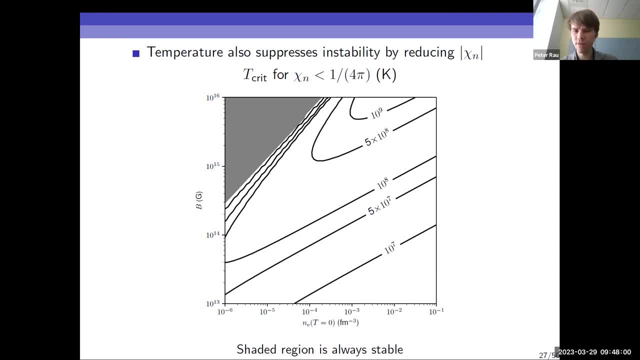 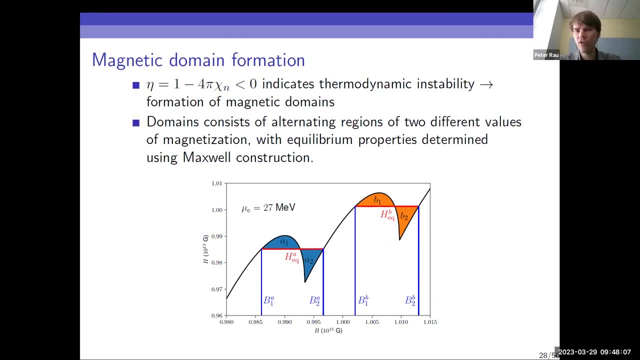 So this sort of shows how the temperatures are suppressing any sort of unstable effects you could have. So I've been sort of dancing around here. So I've been sort of dancing around here, been sort of dancing around this topic, so let's actually talk about this in some detail. magnetic: 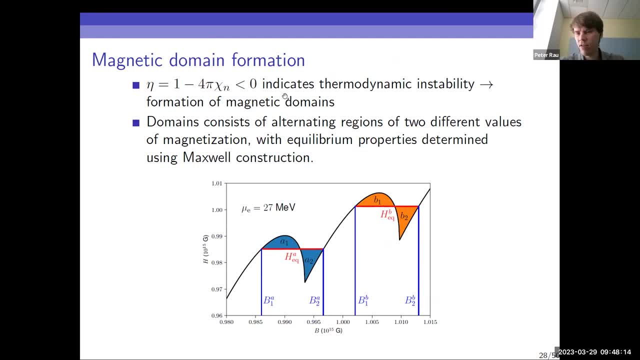 domain formation. so eta being negative indicates the onset of a thermodynamic instability and that is resolved by forming magnetic domains. so what happens is that you have regions of alternating magnetization where you have a fixed h field which form and their properties are determined using the Maxwell construction. so if we imagine a region of, let's say, the crust, which has a uniform 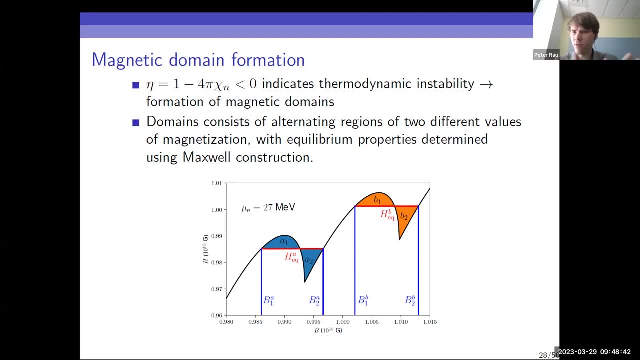 density and a varying magnetic field. it varies like maybe slowly across it continuously. the h field will undergo oscillations with respect to b, but some of those oscillations or some of those regions will be unstable, and so the resolution is that you have regions of uniform h. 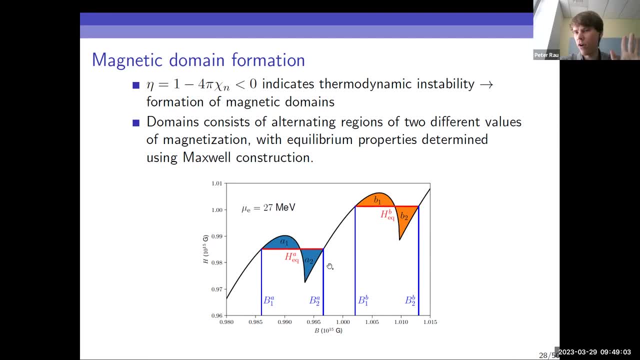 such that the area above and below this curve are equal. so you'd have a region where h is growing uniform, growing uniform, etc. as you move to higher fields. visualizing this in an actual crust which has a density gradient and a, you know whatever field configuration, is quite complicated but you can imagine that. 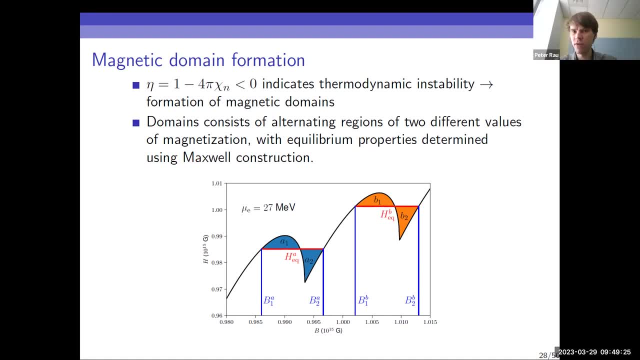 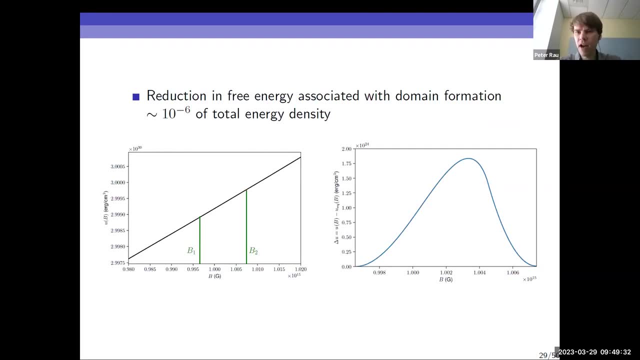 every few meters or so. if you had a sufficiently strong field, you'd have one of these domains being formed. the formation of these domains is accompanied by a reduction in free energy, which is fractionally very small compared to the total energy. so it's around a millionth of the total energy density. it's very hard to see it if you just plot. 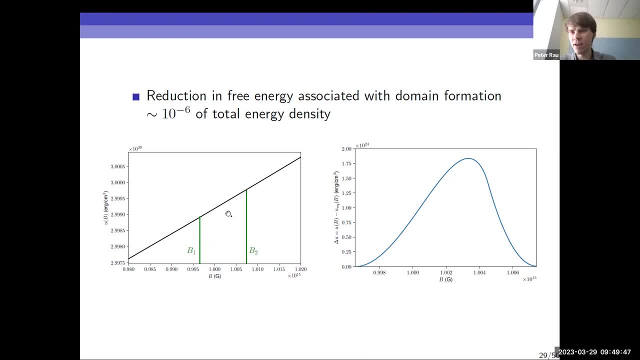 the energy density before you form the domains and after. but if you plot the difference you can indeed see that you have this sort of like bump in excess energy that you sort of liberate by you minimize this energy by forming the domains, because this is excess, is not there. 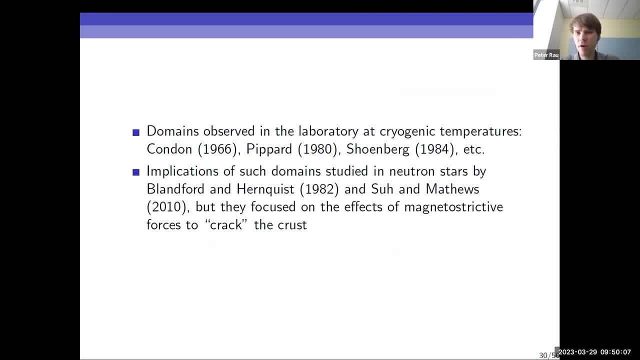 so these domains have been observed in condensed matter experiments at cryogenic temperatures for a long time, but in the implications for them in neutron stars have been discussed by some different authors. but they focus mostly on the effect of magnetostrictive forces. those are forces due to this magnetization field to crack the crust. so i'm looking at things in a slightly different. 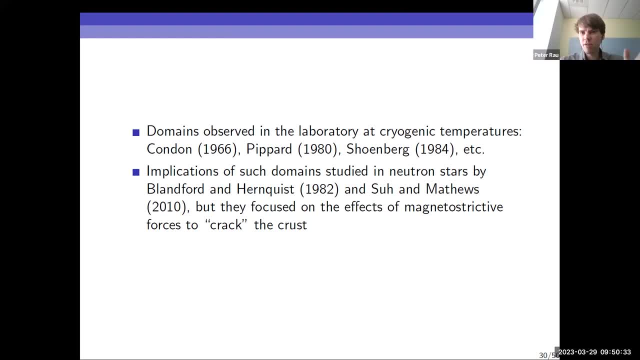 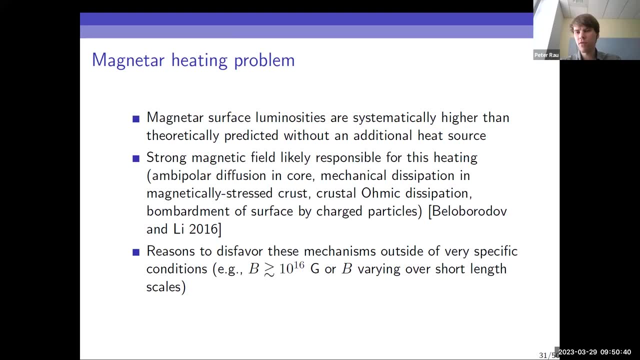 manner. so my idea is: could it have something to do with, uh, heating perhaps? um, so, uh, there is a sort of well-known problem with magnetars in that their surfaces are seem to be too hot. um, they're systematically hotter, so we know that they have a systematically higher surface. 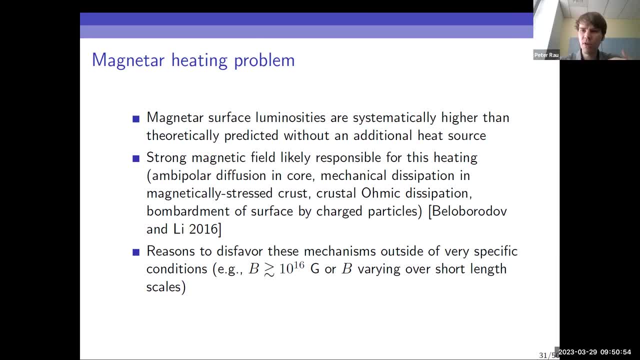 luminosity than um predicted, um, without what you'd have with an external or some sort of internal heating source. uh, it's, you know. believe that the magnetic field has to be responsible for this, because it seems to be responsible for everything interesting that happens in magnetars and there are a variety of different mechanisms which have been studied, which could 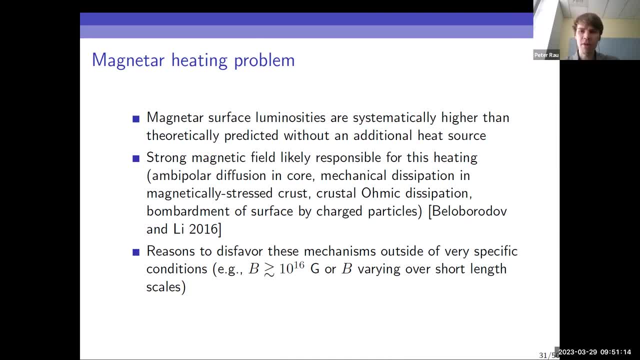 explain, um, this extra heat, um, but there are sort of a few reasons to disfavor some of them. so they require very strong fields, um, and also the fields need to change over short length scales so they can't be smooth, which is, um, something you'd expect these sort of uh, if you had like. 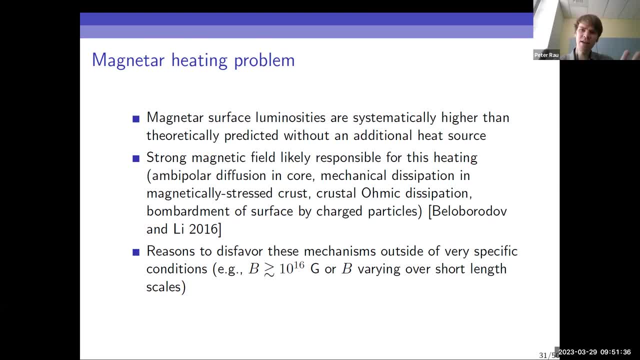 very uh like tangled, not smooth, fields. they might uh decay very quickly um in the early stages of the star and through most of the lifetime, you'd expect them to be um smoother, and because this heating manifests itself at you know time scales, of you know thousands to tens of thousands of years. 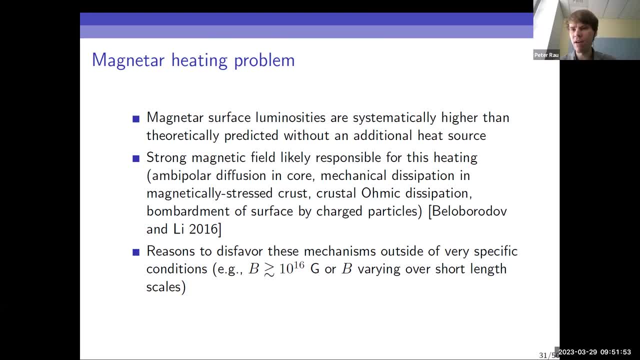 um, it's sort of a question of if you could have this. um it's maybe a very strong ohmic heating in the crust at later times, uh, through such a mechanism. uh, it's not really very powerful, but it's a very, very strong energy issue. it's a very, very, very 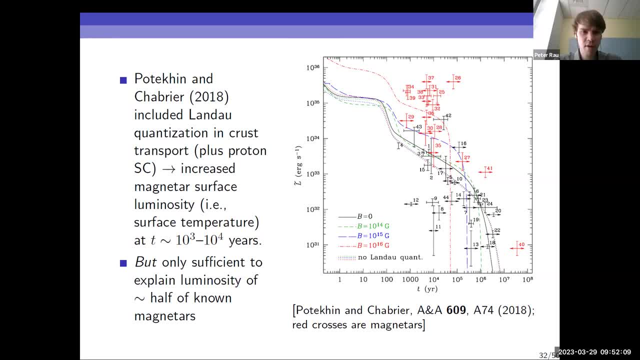 strong and very, very important to have. so, um, the ones that are risk-free. it's the kind of energy with which you put a layer of water to the surface and then you have a heat wave which you have to use in order to make sure you have that. so that's what this topic is about. 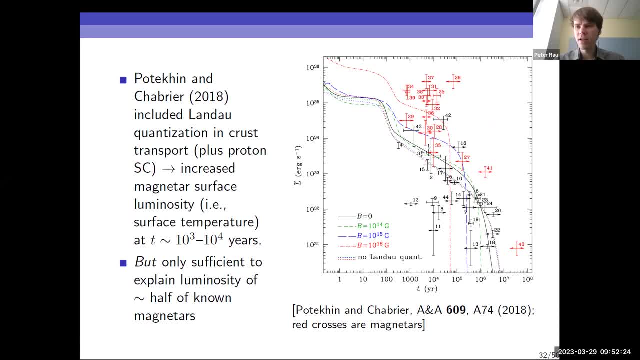 the next slide. so one paper which has studied magnetar thermal evolution and incorporated landau quantization to outer most layers of the star, what's known as the, the envelope um, and they found that um including these lando quantization effects, can uh quite dramatically increase the uh surface luminosity. 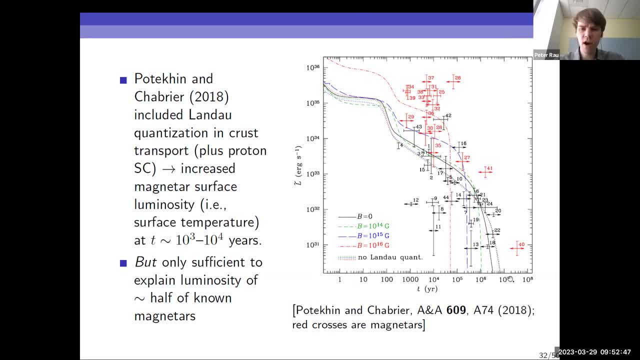 um, and so this is a surface luminosity redshifted as a function of time. uh, the zero field result is in this black line here, um. the results with lando quantization included at different fixed field strengths are shown by these dotted lines and or sort of dot dashed lines, a mix, and if they 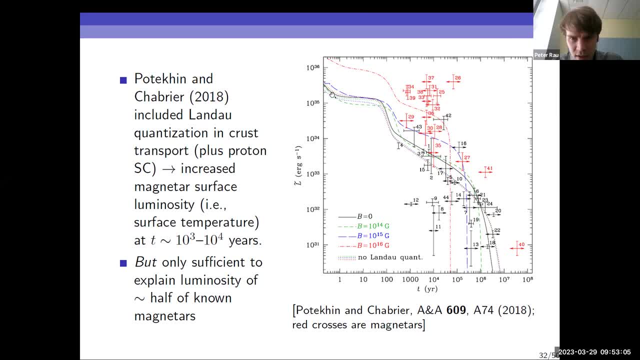 include the fields, but no lando quantization. they get these uh the series of uh dotted lines, uh sort of mostly below the black line here and we're trying to reach these uh red, uh crosses here which correspond to the uh known magnetars, and you can see that, yeah, they're, you know. 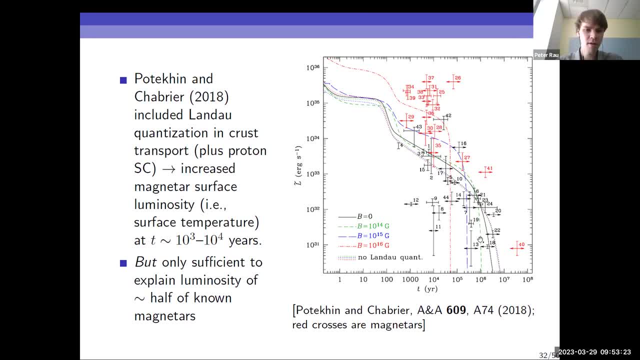 systematically hotter than the non-magnetary neutron stars. um, but what they've included wasn't sufficient to explain the luminosity of the hottest magnetars, and they of course they didn't include a heating mechanism. but they also assumed something unrealistic: that the field doesn't evolve and that it's just like. by this field they mean a. 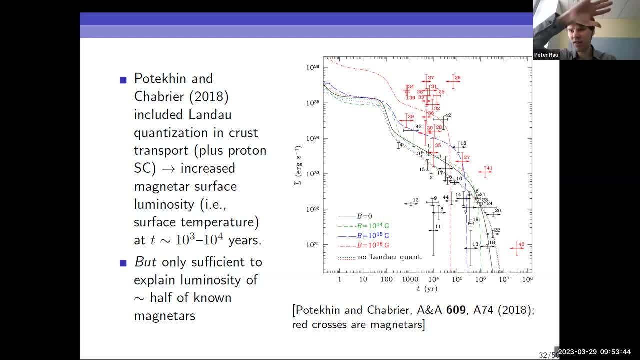 magnitude. there's a, b. the magnitude of b is the same everywhere in the star, which is of course not realistic. neutron stars do have, you know, a magnetic field that has a new direction too, and it's not going to be uniform, it's not going to move um. 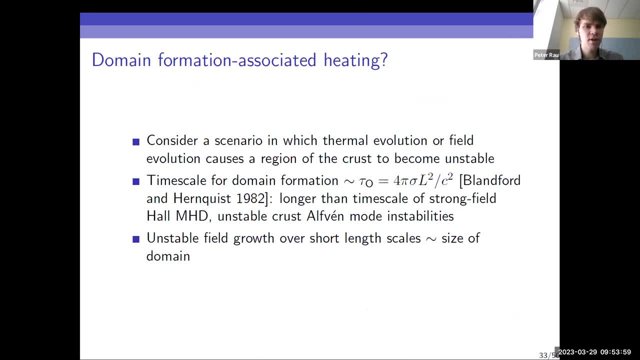 not undergoing dissipation. so my question is: um, you know, is there some sort of mechanism associated with land aquatization that could be responsible for some heating here? so the first i looked at was domain formation associated heating. so, uh, if you consider a scenario where you have a bunch of stable domains but then you have some sort of disturbance like magnetic field, 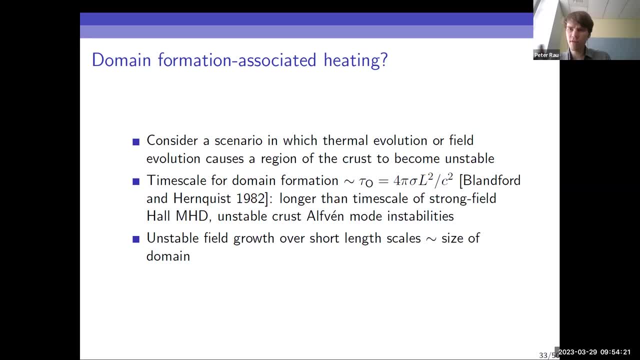 or temperature evolution which causes regions of the crust which were previously stable to now be unstable, to domain formation. time scale for the domain formation is of order, the ohmic decay time scale, which is longer than the time scale of the um, uh, mhd, instabilities in the crust, and so you can potentially have very 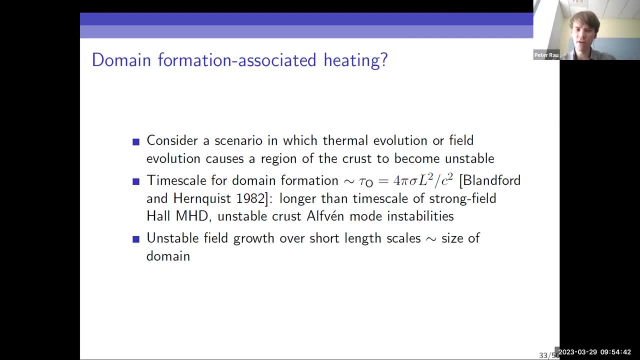 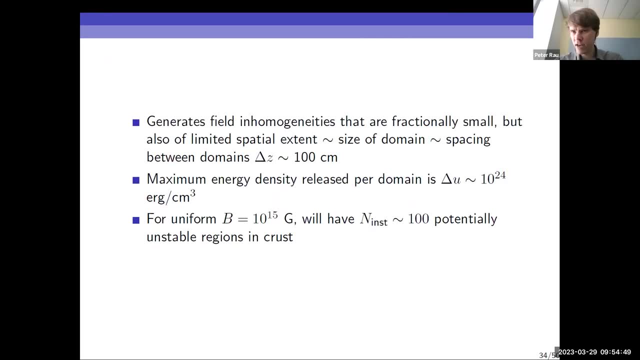 you know, brief duration, uh, growth of field which is powered by the energy you liberate by forming a domain. so, um, these field inhomogeneities would be fractionally small, but over, uh, small length scales, over the length scales typical of domain sizes, so maybe like meters or so, and let's say you're liberating maybe 10 to the 24. 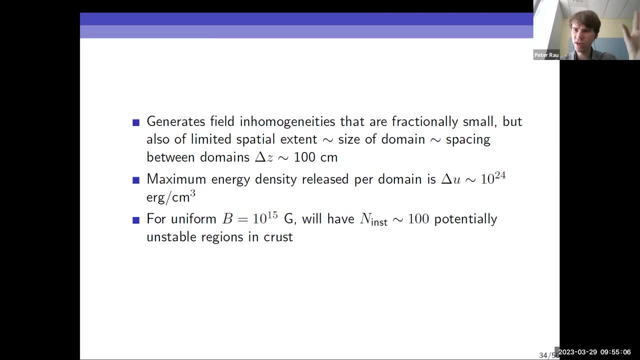 uh bergs per centimeter, cubed in sort of uh energy density, and you have these like maybe shell, like domain structures which are being formed. um, if you have a uniform, let's say, magnetic field of 10 to the 15 gauss, you'd have about 100 of these essentially unstable regions. 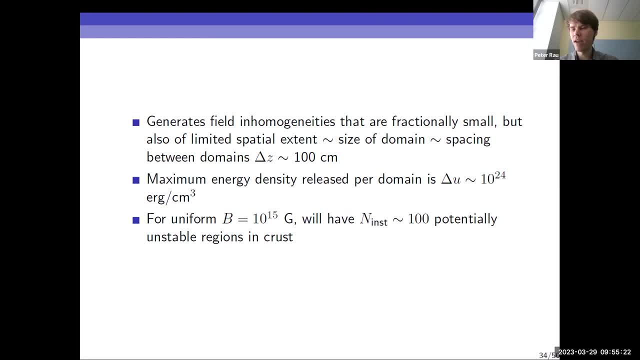 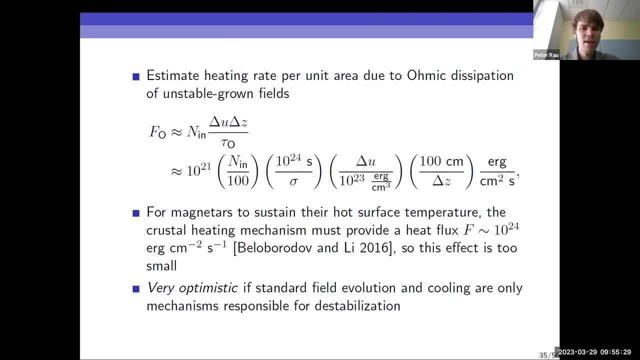 maybe being active at once, and could that give a, you know a heat flux that would help um keep these uh temperatures uh higher. and the answer turns out to be not quite uh. so if you estimate what the rate of ohmic heating is from these small scale length, these small length scale fields being 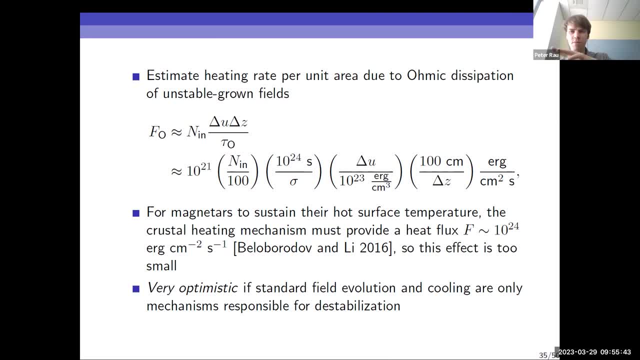 grown unstably from the energy that is imparted to them by the formation of these new domains at different positions. um the flux you get from it is about a factor of a thousand, too small to be responsible for. um providing the heat required to explain the hotter surface temperatures of magnetars and 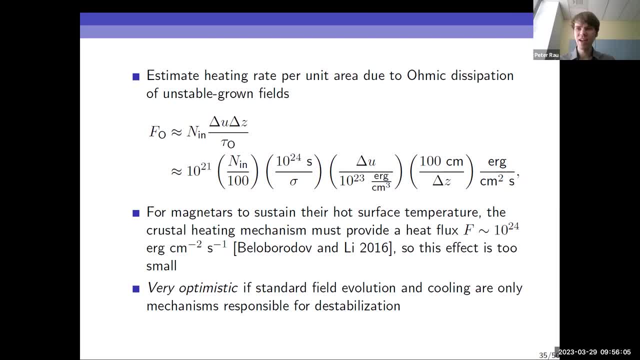 additionally, this scenario was very optimistic anyway, because i'm assuming that all these regions are becoming unstable to domain formation at once and this is sort of repeatedly happening, which is probably not going to do so. it's it's far too intermittent of a process to really be relevant um. 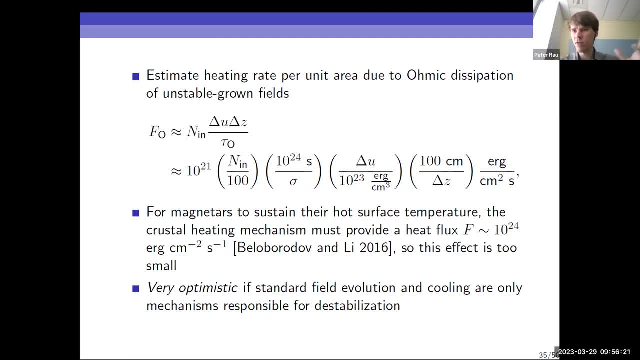 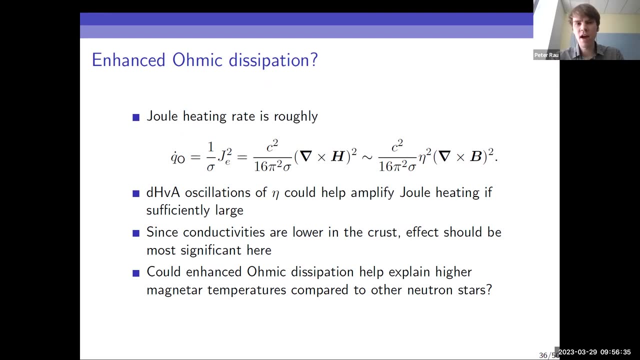 but there is something which is relevant um that relates to lando quantization um that could have some uh important implications. uh. so i'll move on to the sort of final part of my talk now. um, and this is uh enhanced ohmic dissipation, so the joule heating rate um is just j squared over the. 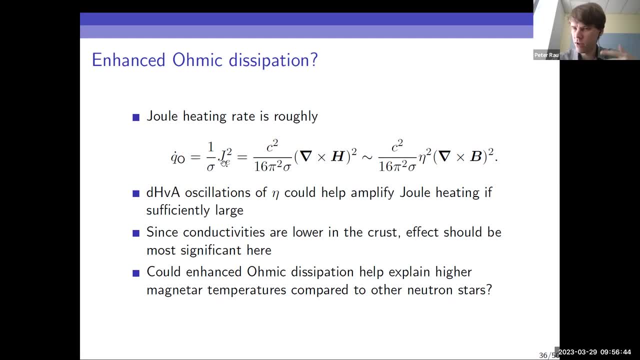 conductivity. but we know that j in you know our case is curl of h and not curl of b and because of that you could um this doesn't quite. you know it's not exactly this, but it's about this: um you get an amplification of the ohmic heating that goes as um the eta differential magnetic susceptibility squared. 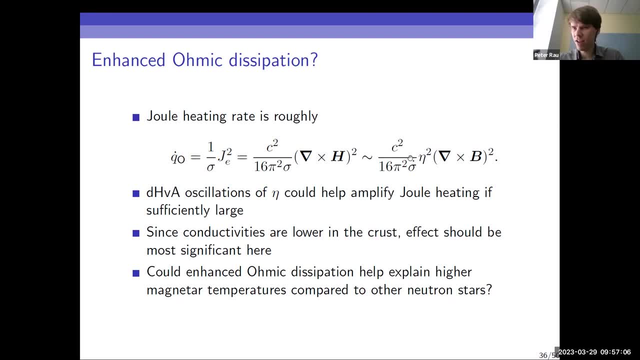 and even if this can never be negative, because you'd have domains being formed that would, you know, make you thermodynamically stable, you could have large oscillations of this that could give local amplification of the heating rate. um, so again we're looking at amplification of heating. 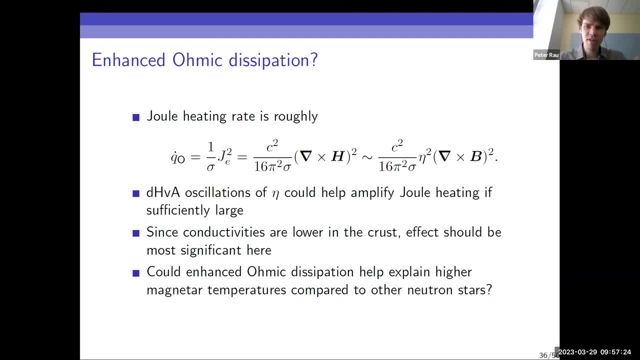 because of the haas fan alpha in oscillations. but since the conductivities are lower in the crust, we want to look at what's going to happen in the crust, um, because of course you have this term in here, um- and our question is: could you know this? enhanced ohmic dissipation, help to explain? uh. higher magnetar surface temperatures. 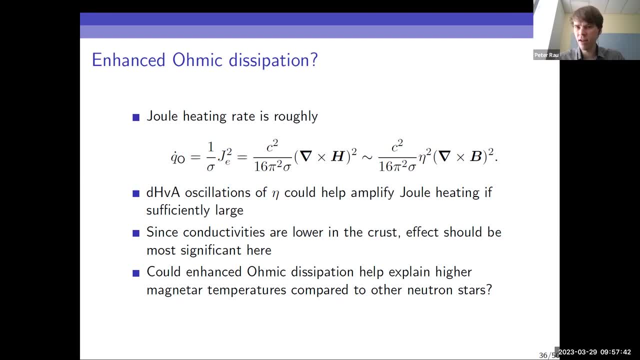 because another thing this will do is generate field inhomogeneities, because these oscillations occur at different points of um, like it's not spatially uniform quantity, so you have regions which are decaying faster than others. that helps generate field inhomogeneities and additionally, this current appears in the hall term, so you have 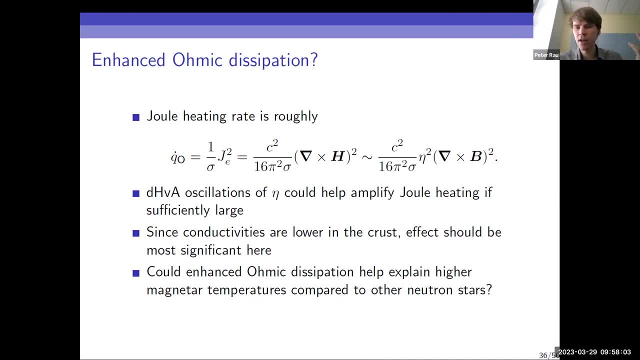 oscillations occurring in the hall term itself. and the hall term actually does something very interesting, um, in magnetic field evolution, which is that it generates a. if you start with a purely poloidal field, it will generate a toroidal field by itself. so, um, it has this effect of generating. 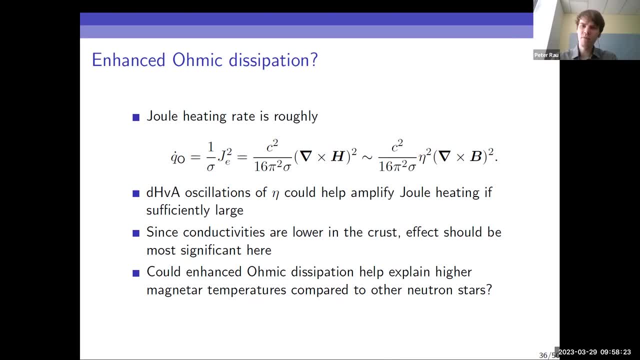 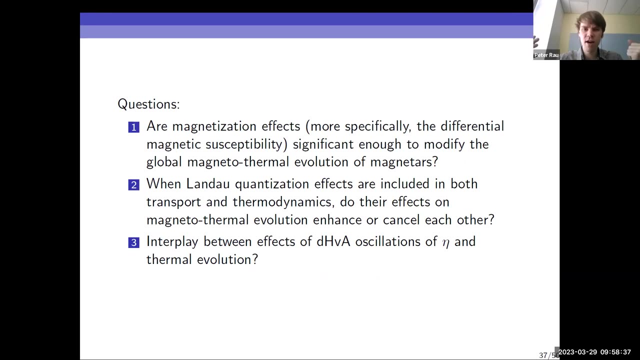 fields like transferring energy from one field to the other. but because you have these oscillations in it, it could do so in a way which creates fields with with more small scale structure, which are more susceptible to ohmic dissipation. um, so, just sort of review these questions, um, we 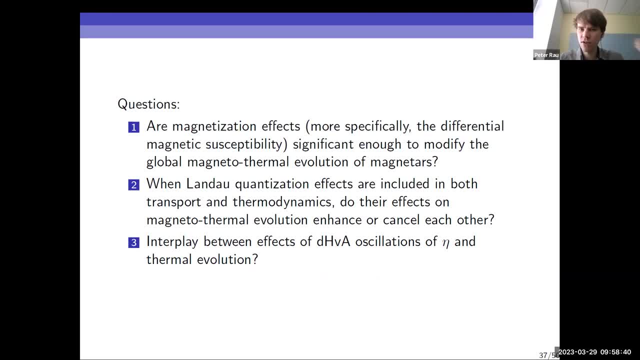 want to look at the significance of magnetization effects to magnetothermal evolution of magnetars, if you include the effects of both magnetization and the uh oscillations of the uh transport properties due to these effects. add or do they cancel? do they work against each other or not? um, and what's the? 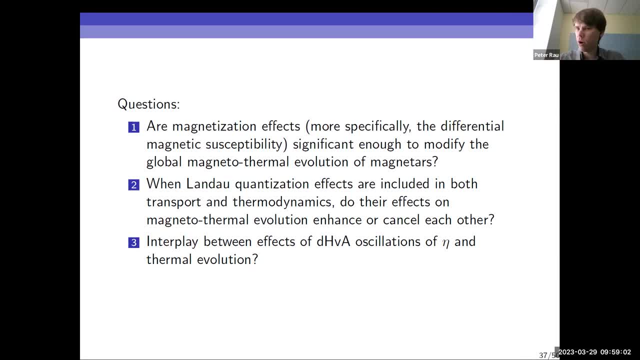 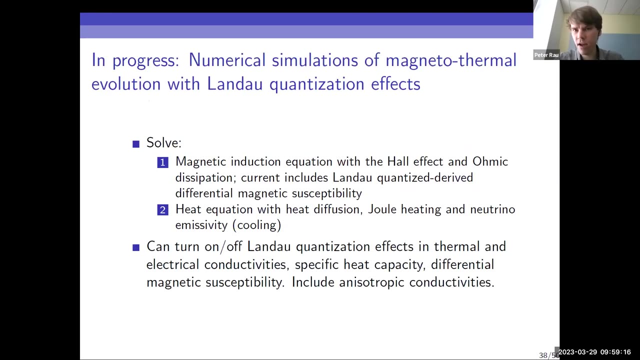 interplay between the evolution of um the land, of quantization effects and the temperature, because we know that higher temperatures suppress these oscillations. so when do they become um important in the lifetime of the magnetar, essentially. so i'm going to report on some in progress uh simulations. 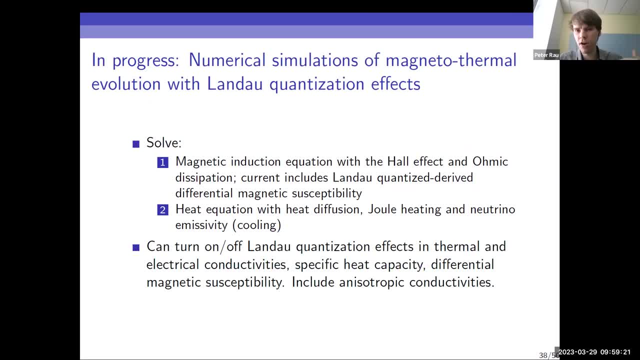 of uh field and temperature evolution of magnetar crusts with lando quantization effects included. we're solving two equations: uh, the magnetic induction equation, um, so we have the hall effect and ohmic dissipation in there. so we're assuming that the crust is um rigid. essentially, 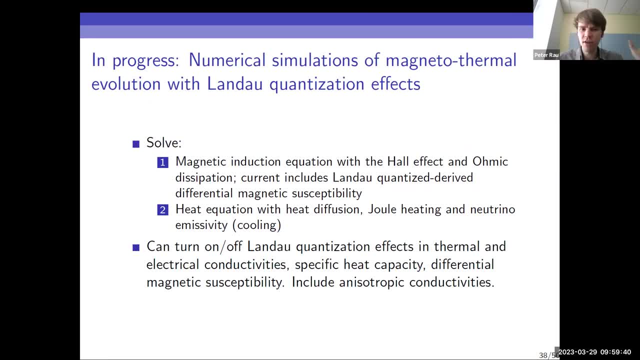 um. so the current terms will contain lano quantization, derived differential magnetic susceptibilities. so that's going to give us some interesting effects. um, in addition to the lando quantization in the connectivities, and we have the heat equation, uh, which includes heat diffusion of. 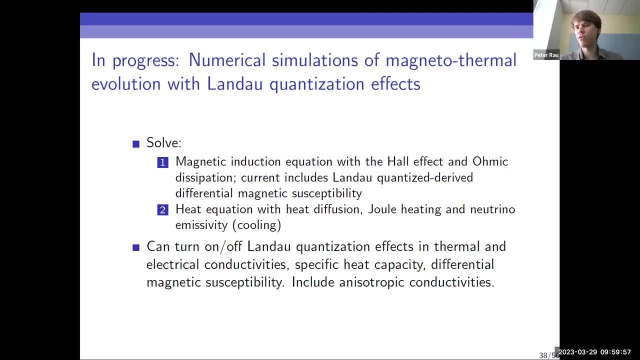 lando quantization effects, so we have a sort of realistic temperature um evolution. we can turn on and off lando quantization effects in the conductivities and in the thermodynamics, by which i mostly mean the magnetization and its differential um components separately. and when we include lando quantization effects in the conductivities we also 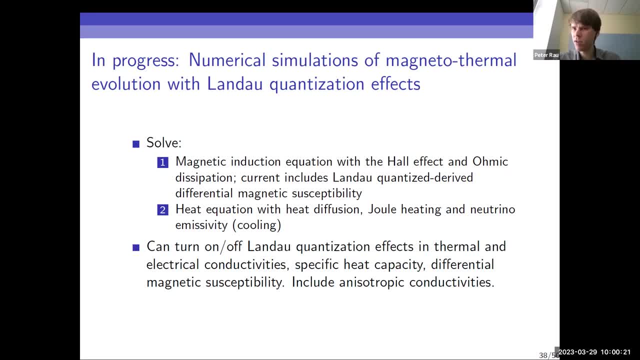 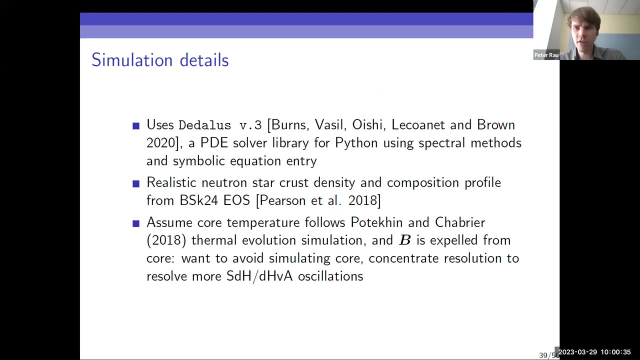 make those conductivities anisotropic. so the components of the conductivities parallel and perpendicular to the magnetic field are distinct. so, um, the simulations have been run using uh, a python pd solving package known as dedalus, which uses spectral methods. uh, we are again focusing on 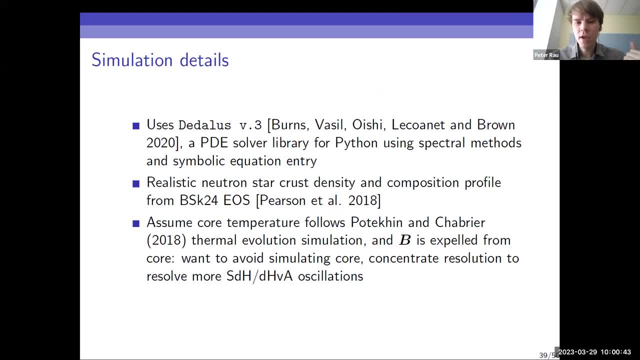 a crust which is generated from the bs k24 equation of state, and we're assuming a few things to make our lives easier. we're assuming that we can take a temperature profile uh from the the core evolution of the trust core uh in thebiorian literature that shows that the crust core boundary is at a. 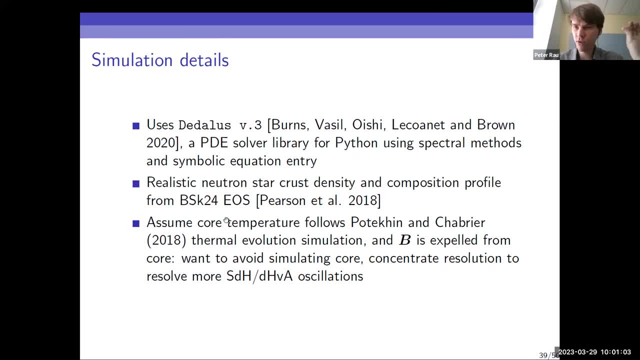 temperature computed by somebody else, um for a. essentially the exact same equation of state that we're using um, but there could be some um maybe problems with doing this, but it should give a somewhat reasonable estimate of um, the inner temperature at the crust core boundary. and then we're assuming that also the field does not penetrate into the core, which is more reasonably. 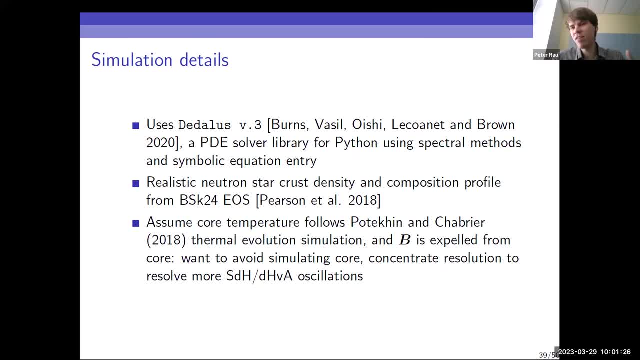 that's something which is often assumed. it may not, you know, cover the core, you know, but it's not exactly be correct with magnetar strength fields. but it's essentially equivalent to assuming that the core is superconducting. So we're looking only at the crust, and doing this allows us to. 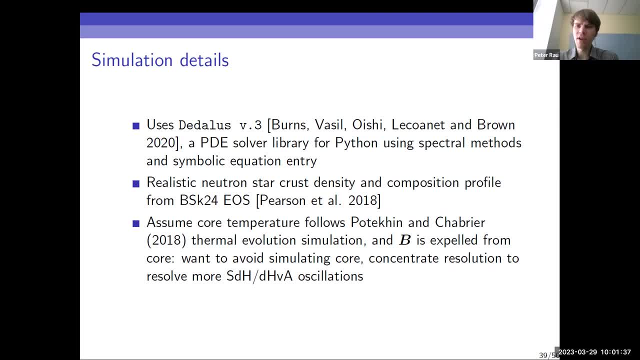 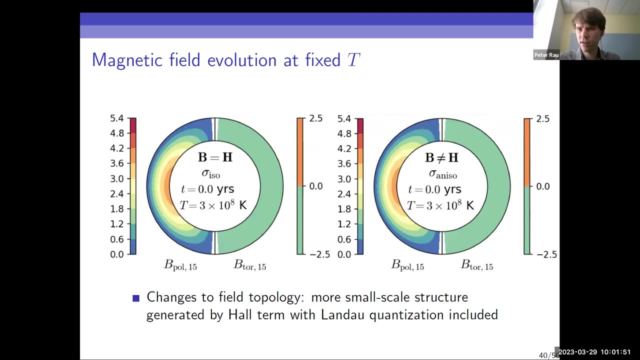 focus our resolution in this crust and to capture more of the oscillations of the Lando quantization-based quantities. So the first simulations I will show are magnetic field evolution only done at fixed temperature. So this is around 3 times 10 to the 8 Kelvin. 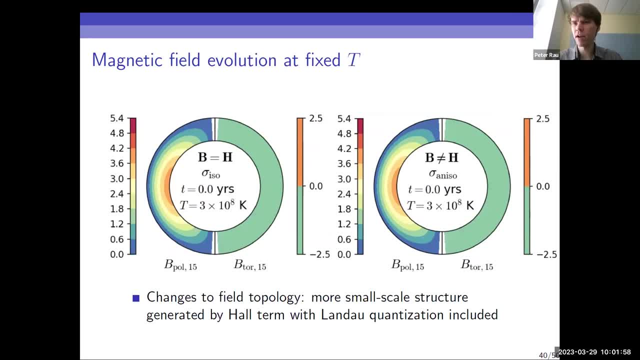 typical temperature that you get after around maybe 1,000 years of magnetar evolution. On the left we have simulations ignoring Lando quantization entirely, and on the right we have ones where we're including it in everything. So it's B not equal to H magnetization. 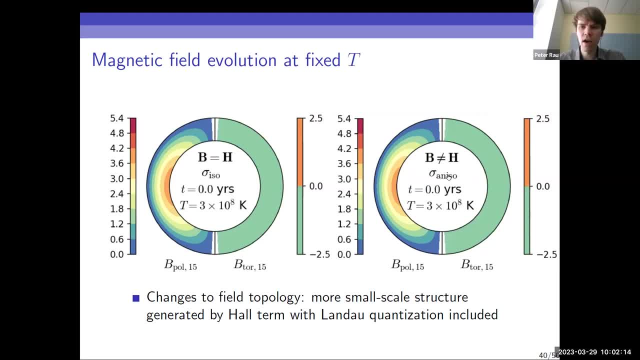 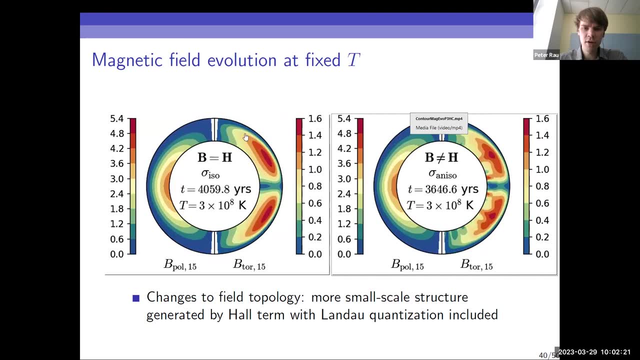 in there and also Lando quantization in the connectivity. So if I run the simulations now, the main thing to note is that you get a toroidal field generated from an initially purely poloidal field. So the poloidal field is on the left. It doesn't really evolve that much. I mean it's slowly decaying due to. 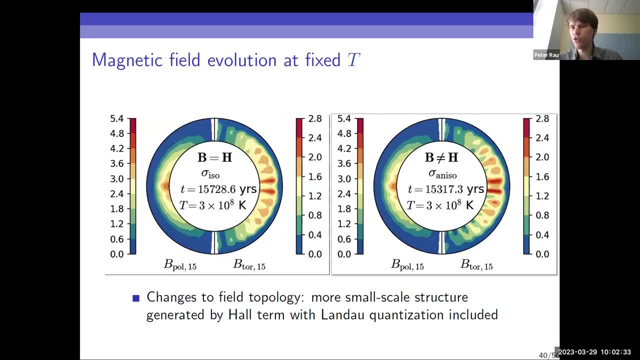 moment decay, but also transferring energy into the toroidal field which is being generated. But the thing to note is that the toroidal field which is generated on the right has much more small-scale features and sharper small-scale features than the toroidal field on the left. 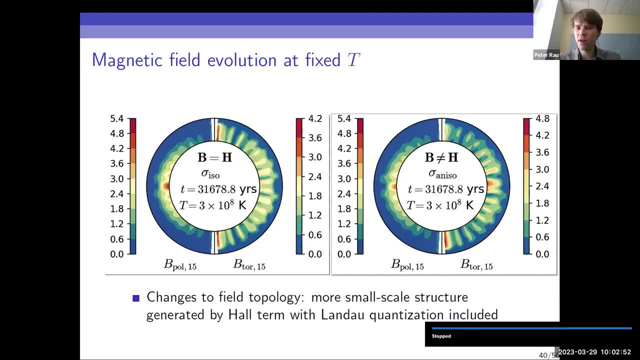 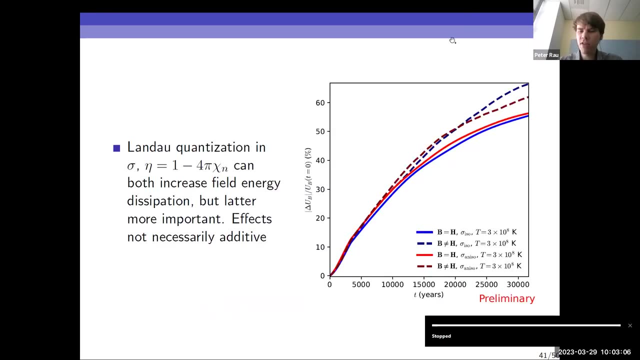 And that is because you have these Lando quantization-based differential magnetic susceptibilities in the current, which help to generate smaller-scale field features and also actually help to dissipate field energy more efficiently. So if I look at the next slide, this is just plotting the 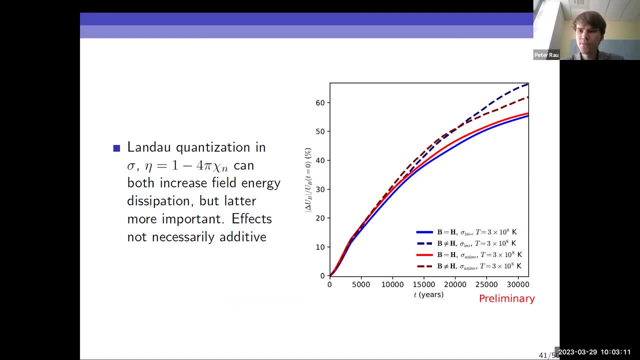 percentage of the field energy dissipated with time for four different configurations, two of which I showed in the previous slide. So the solid lines are configurations where you don't have the magnetization, And then the different permutations of the odd activities. and the dotted lines- dash lines- are those configurations where you include Lando quantization. 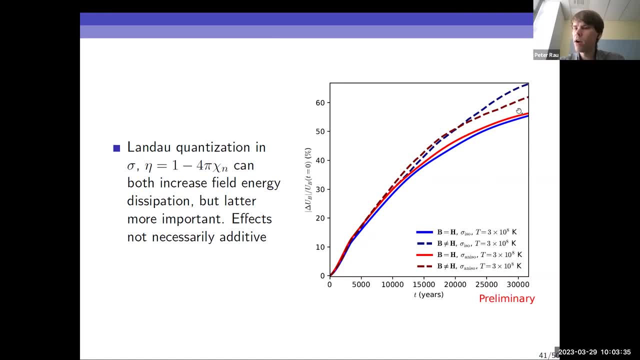 and magnetization And you see that those ones give systematically more energy dissipated at these temperatures. It's, you know, maybe 25% more than the case where you ignore the magnetization entirely and both of the lando quantization effects. 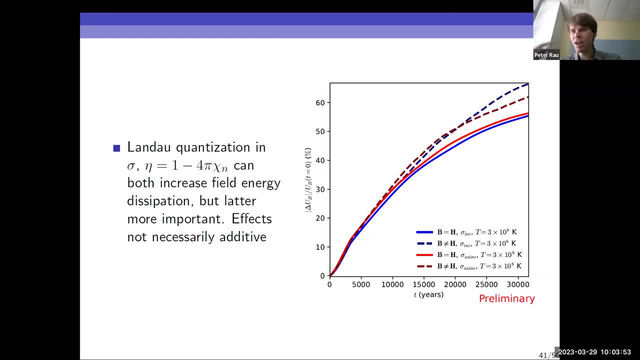 Okay, increase field energy dissipated, but the magnetization tends to be more significant and the effects are not necessarily additive because you get these oscillations in the connectivity. so the regions where maybe it's, uh, lower or higher than it, then you know it's not. 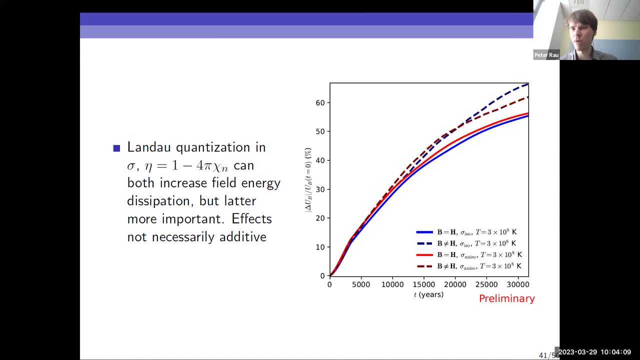 uniform anymore, and so you can. you know, you have to be a bit careful about saying that you're always going to increase the dissipation, um. one thing that is interesting, though, is, of course, what happens if you go to lower temperatures, because we know the oscillations should be more significant. 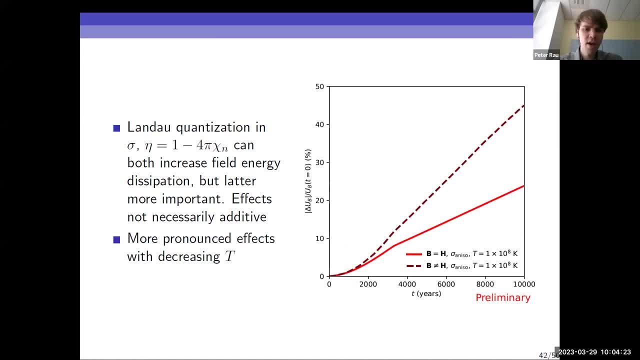 there and you can get you know markedly increased dissipation um. so this is comparing two simulations, both of the same conductivities, but with not including magnetization in the lower line and including it in the upper line, and you essentially double the amount of energy being dissipated after you know a time scale around 10 000. so it's very important um at these lower. 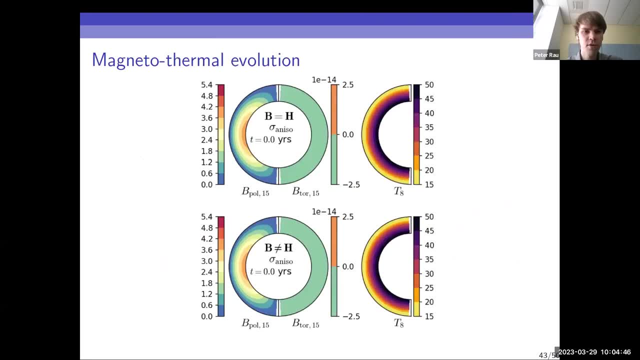 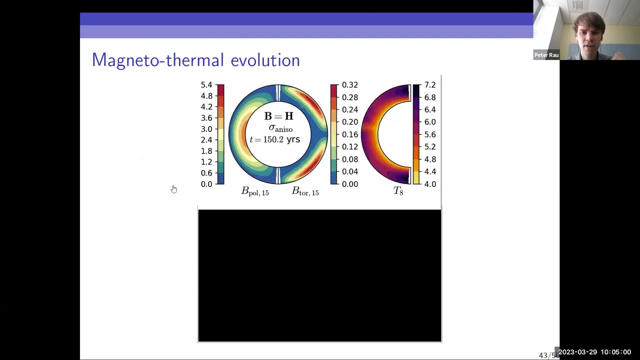 temperatures, and so, finally, i'll uh show some evolutions where we evolve both the temperature and the field. so on the top we have a simulation without the magnetization. on the bottom we include it and we have anisotropic conductivities in both, and the thing to really focus on here is that, initially, 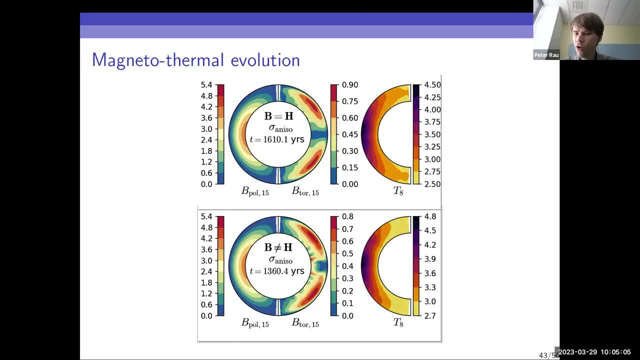 the evolutions are very similar of the toroidal field, but later, once you get to lower temperatures, the toroidal field starts developing much more small scale structure. it's not exclusively an l equal to spherical harmonic uh toroidal field like it's. it retains this feature, um essentially. 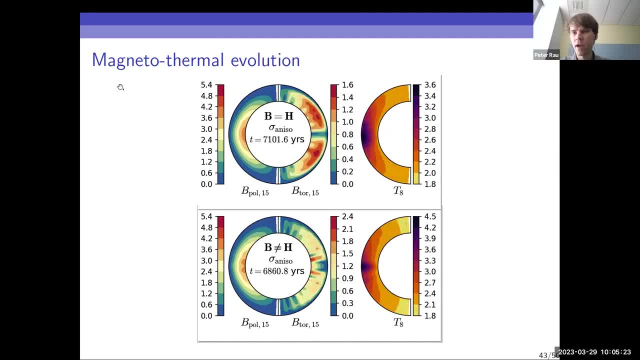 and so we're going to get to all of these in just a second. but to the next slide, um. so this is also a really important the uh ansch action parameter, which is kept in mind for almost the entire evolution for um. the case where you ignore the magnetization um, and i'll note that this uh hot ring feature um at the equator of the 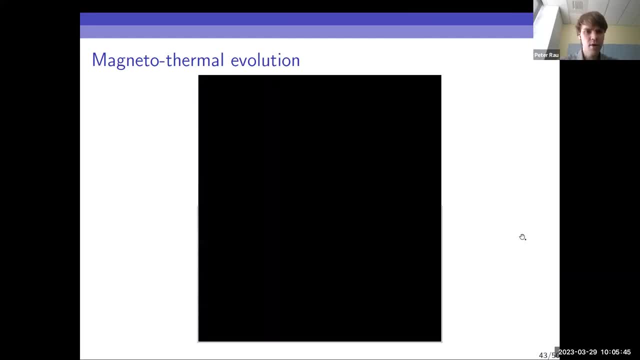 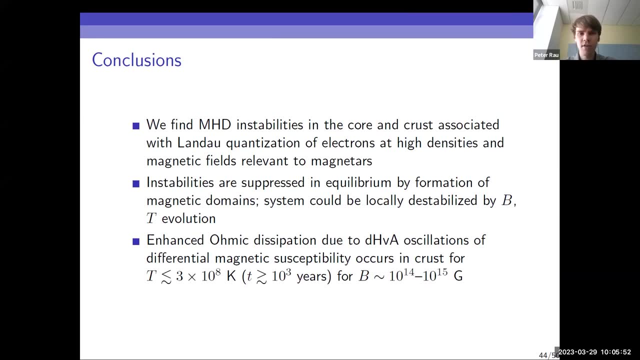 neutron star is something which has been observed by other calculations of which do magnetothermal evolution of neutron stars. uh, so this is- you know, not just us getting this uh feature here- and the crust and core of neutron stars associated with Lando quantization of electrons. 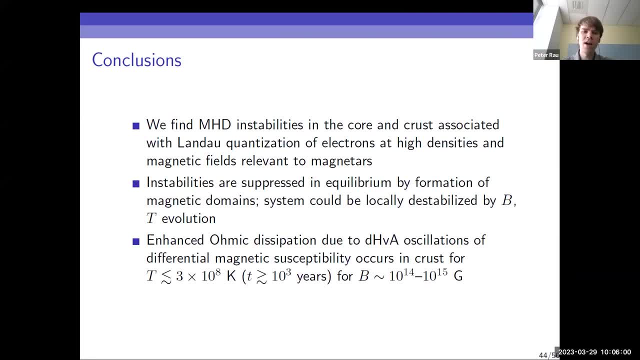 The instabilities are suppressed by domain formation, but they could be destabilized by later field and temperature evolution. And maybe of most fundamental interest is that we can find that if you account for this Lando quantization-induced differential magnetic susceptibility in a field and thermal evolution, it will enhance ohmic dissipation. And this occurs at sort of 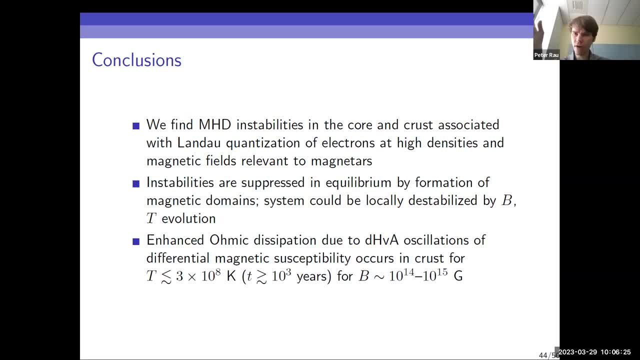 times and temperatures relevant to where our heating curves are sort of mismatched with what we predict if we don't include the heating at all. And again, this is of course all very dependent on the field strengths and not so much on the initial temperature, because as long as it's sufficiently, 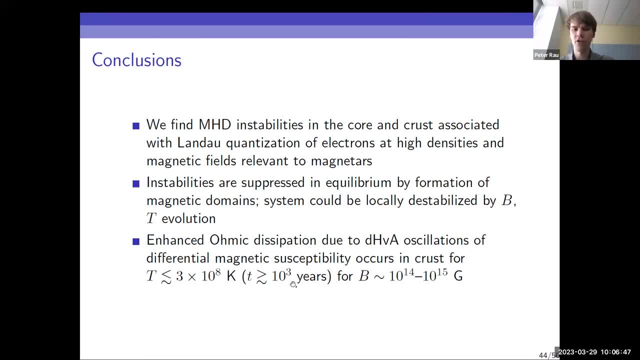 hot, it's going to be a little bit more heat-sensitive And so, again, it's a little bit. you tend to reach the same cooling curve in a very short period. So yeah, with that, I will thank you for your attention and take any questions. 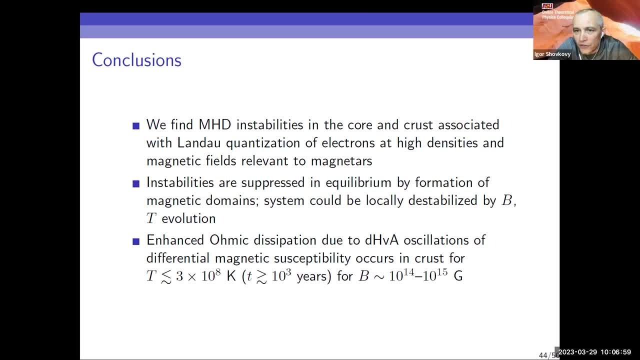 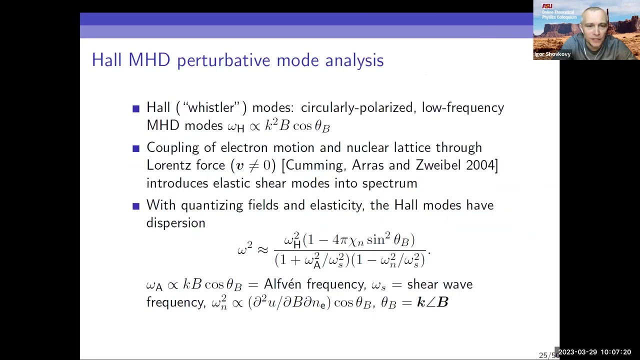 Thank you so much for a nice presentation. Now let's go to questions. If anyone has any questions, please use the raise hand feature. Let me see. Actually, I have maybe a simple clarifying question so that I understand it right On page 24, I really misunderstood one statement that you made. 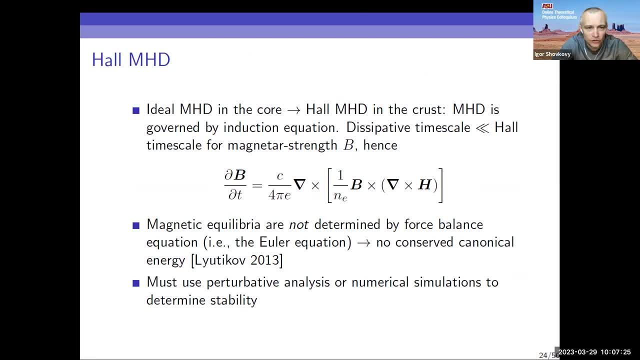 here It says dissipative timescale much shorter than whole timescale. If that were the case, that means that dissipation happens too quick. It's the other way around, right, It's the other way around. Yes, Yes, Oh, okay, Good. 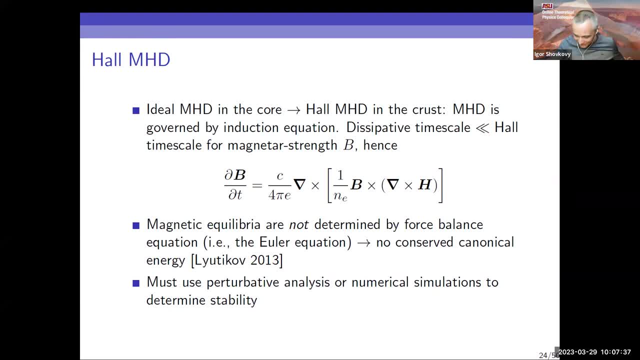 It's definitely the other way around. Yeah, Because I thought I really lost my mind. No, no, Yeah, yeah, no, Okay, good, Another simple, very simple clarification, Clarifying question on page 32.. There were some labels, numbers, next to the points. 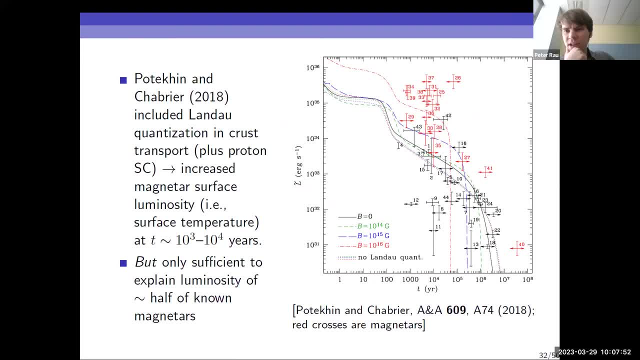 What were those? I think those are just. they have a list of stars and it just comes from that. I don't think in this paper, but in a related paper they have a table which shows the phone numbers for all of these stars, right? 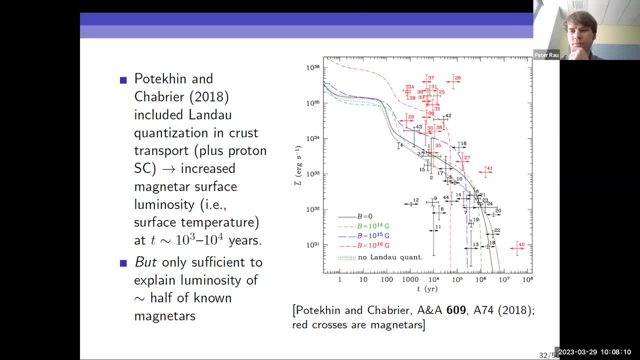 Oh, okay, Okay, I get it. Okay, Yeah. Anyway, we have a question from Henry De Jong. Please, Henry Hi, Thank you very much for a really nice talk Question again about: in the past we've learned about neutron stars and their layers, and 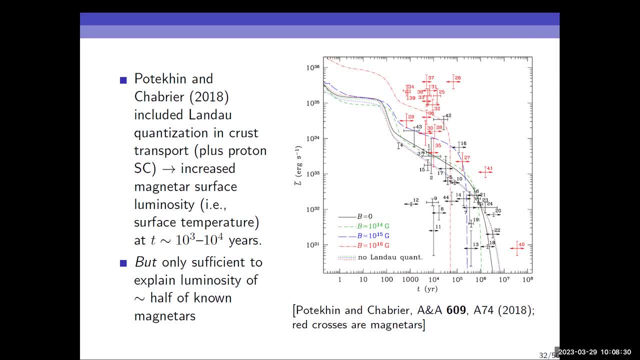 particularly right at the crest and a little bit below, like you have these pasta formations and things like that, honeycombs and so forth. How do you take that into account in your model and how do magnetars perhaps differ from these normal or whatever you would say, nominal neutron star structure? 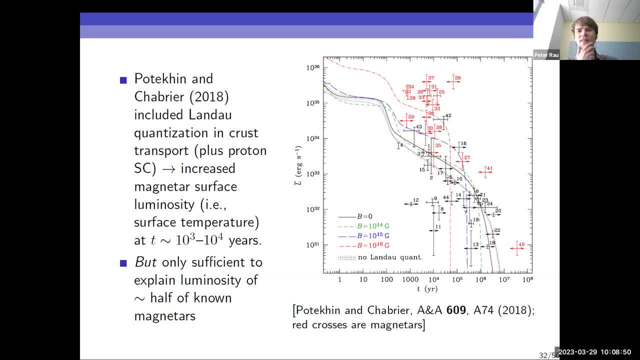 And what do you consider the crest depth? Okay, Yeah, So that's a very good question. I don't account for nuclear pasta phases in my crust. The question of what happens to the nuclear pasta when you have a very strong magnetic field is very interesting. I think there are people who are at least thinking about this. I'm not. 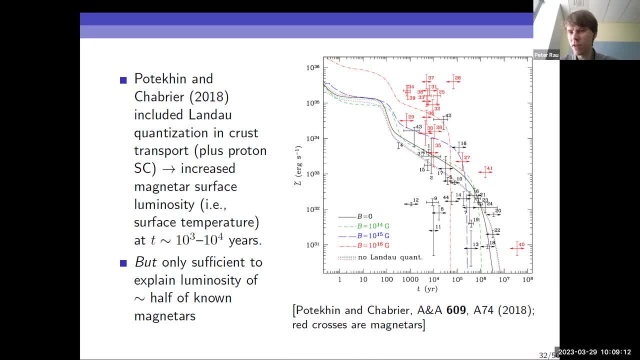 doing it so much, but I think it's definitely something which should be looked at. I am using an equation of state which really doesn't account for magnetic fields at all. Now, I'm not using fields which are high enough for that to make a big difference. 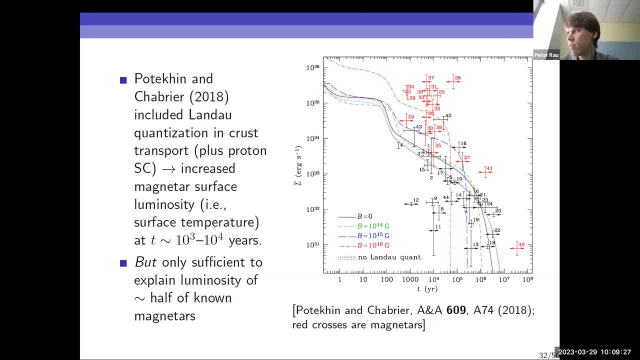 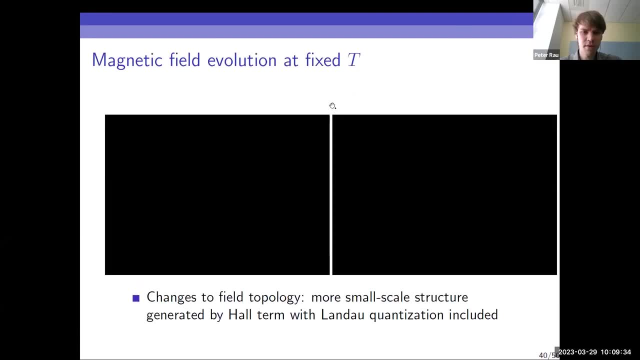 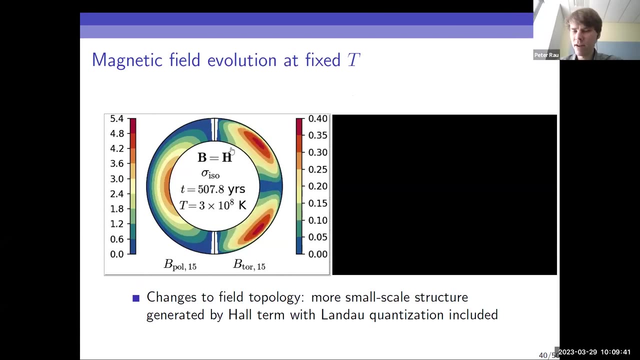 in anything And my crust thickness is: it's not the full, like in the simulations, it's not the full crust. So we can start one of these and pause it. First I'll say that this has been magnified by a factor of four to make it easier to show The thickness of the. 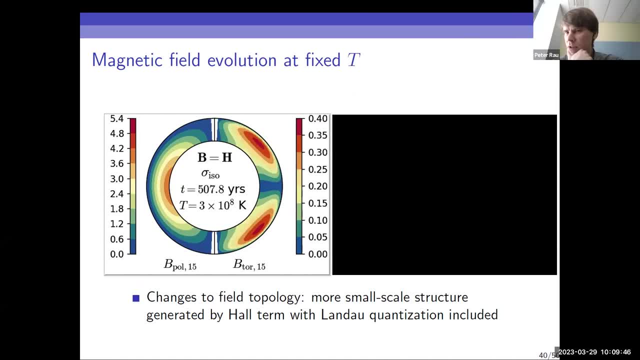 crust is about 800 meters that I simulate And I go from the crust core boundary to a mass density of 10 to the 10 grams per cubic centimeter. So that's a factor of four below neutron drip. I don't go to the outermost layers of the crust, I use a heat blanketing envelope. 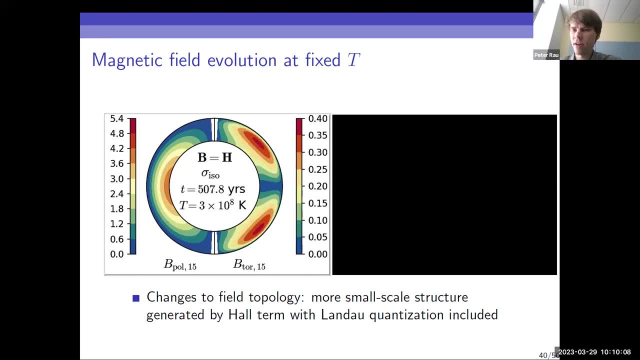 approximation to deal with that and to extract a surface temperature for instance, It's too difficult to do the simulation And all those outer layers, And I guess a follow-up question would be, it seems in that your model then would affect the lifetimes of the magnetars, correct? 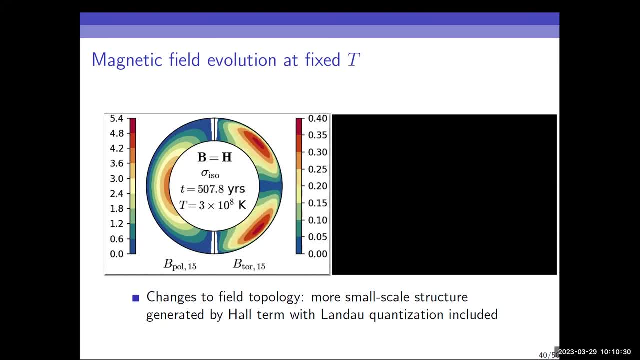 Maybe we can see that in our observations, even though we have a very limited number. Is there any observational evidence to support this? in terms of lifetimes? So it would be. yeah, so I mean, one thing that is actually noted is the life. I mean, if you look at the 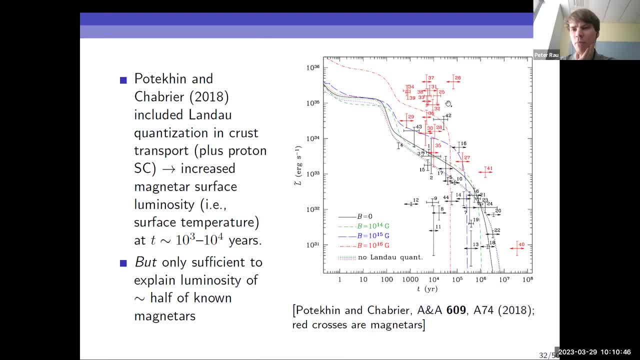 lifetimes. here they do burn out faster, right? So that is one thing that is noticeable. I'm not sure I have any enough precision to say that they should burn out any faster than is predicted. Like I don't have that much detailed information yet to say that this predicts that they do burn. 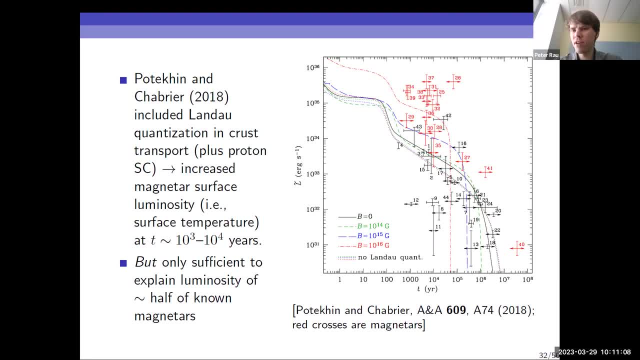 out faster, but the heating mechanism in general, like whatever it is you know, does argue that yeah they, this does shorten the lifetime. yeah, Yeah, yeah, okay, Thank you, Yeah, Okay, any other questions? 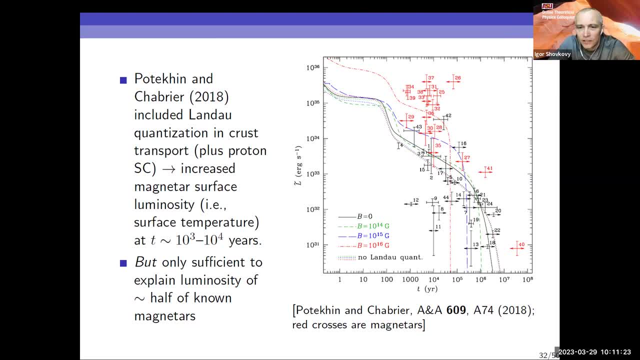 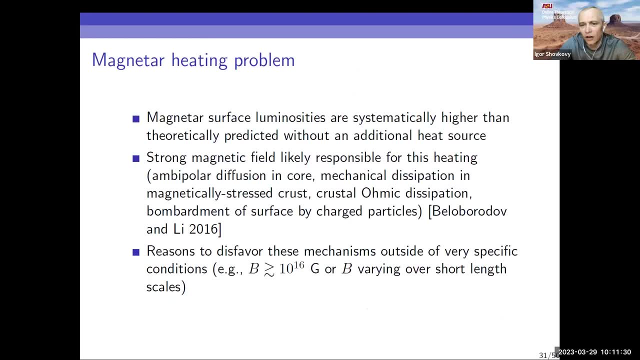 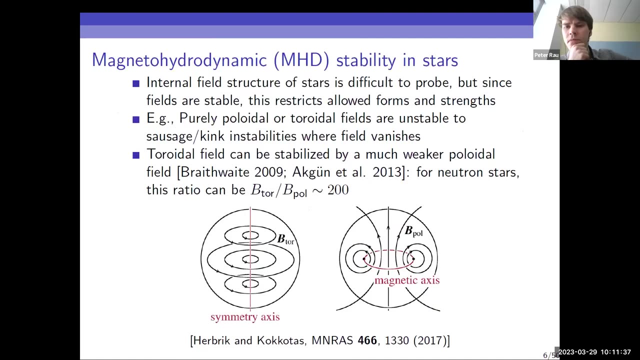 I actually have another simple question. In the introductory part you were talking about the typical scales for the toroidal fields to be a hundred times larger than poloido theoretically predicted, But in your simulations, in fact, I seem to see the other way around. 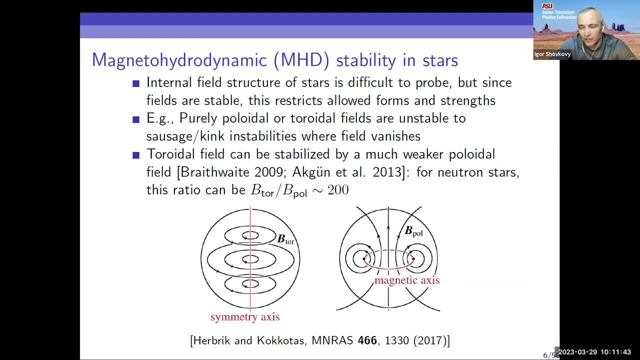 The actual induced toroidal fields seem to be, well, at least an order of magnitude smaller, if not less than that. So, yes, well, Is there a contradiction there? Okay, so I did not include a yeah, so the initial field in those simulations was a purely 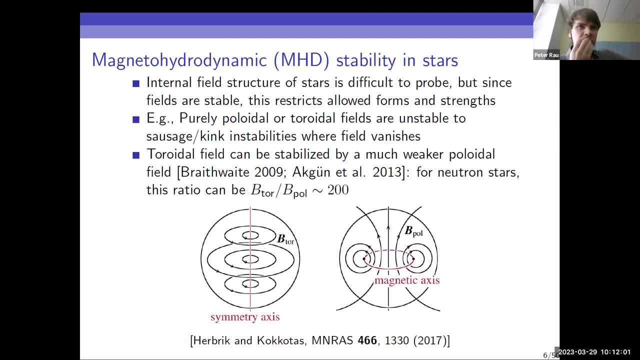 poloidal field, So this would be so okay. so yeah, It's a purely poloidal field, but it's the magnetic field is smaller. It's actually not so small. so if you compare the two, like it's like an order of magnitude smaller than that. 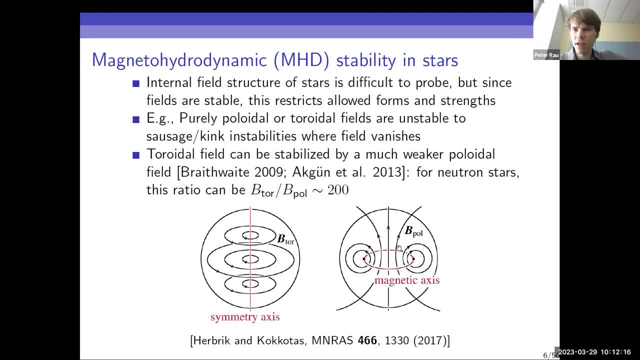 magnetic axes are not in the. they're not in the region where the magnetic field exists. So it's slightly different when you have a crust confined field, which is what I have here. I don't have like. this is assuming the field is existing throughout the star. 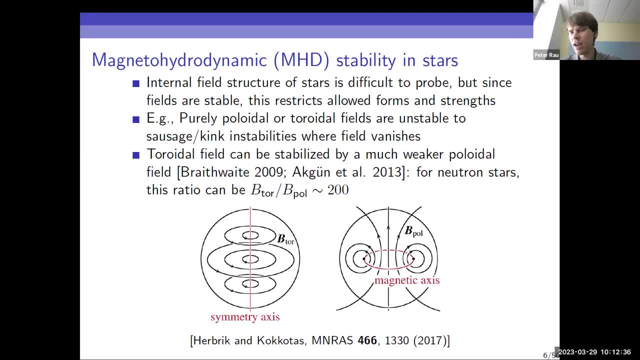 So I do plan to include both a initial ploidal and a initial toroidal field at some point, But at this point I'm not. I'm not developing the instability along any of these axes because, like I, have the ploidal field. 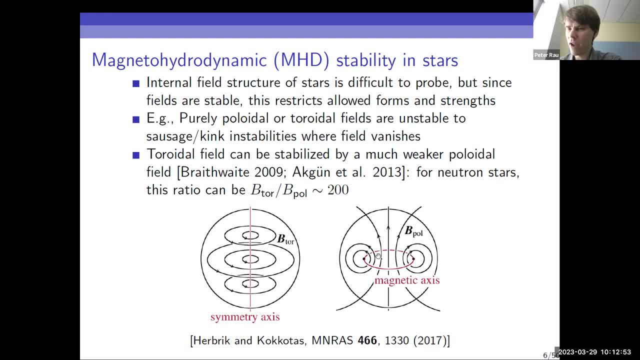 which doesn't have this magnetic axis in the simulation domain, And then it develops a toroidal field, like almost instantaneously. it's quite weak at the start, So it's not really restricted by like these conditions when you have this crust confined field. 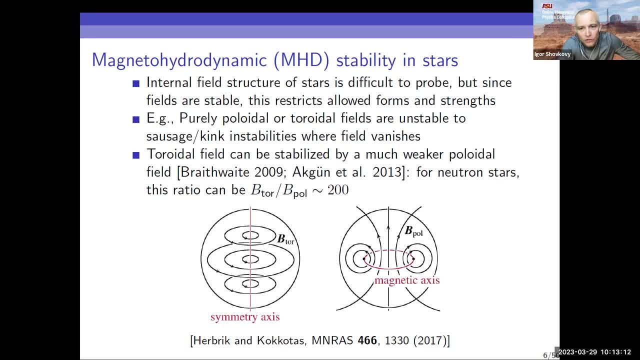 I see, I see. So the geometry of that model essentially is very restrictive to consider this kind of physics. I see, I see. good. And finally, maybe the last question I had related to the hotspots on the equator. hotspots on the equator. 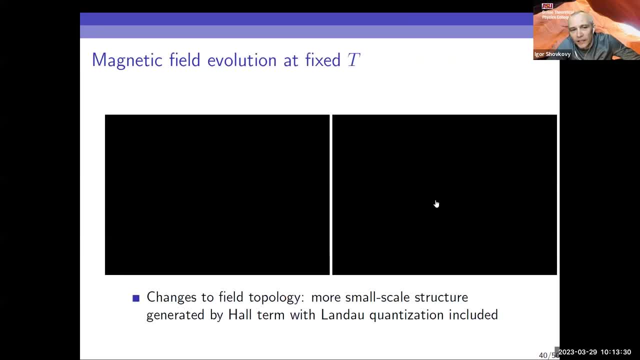 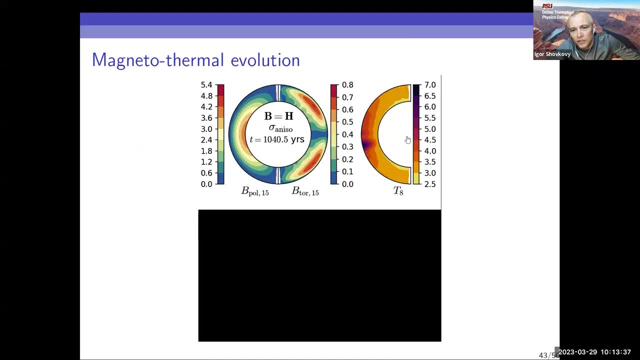 I was a bit confused by that, frankly. One thing that I sort of imagined: that when you have a magnetar, generically the hottest region would be in the core of the star and, because of the much higher conductivity in the direction of the axis of rotation. 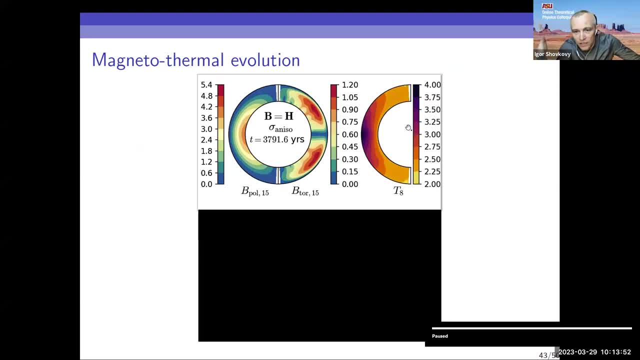 basically along the magnetic pole directions. there will be hotspots because heat will be easily going from the center of the star in the direction where the heat conductivity is the largest, basically along the magnetic poles and not to the equator. And you seem to suggest something else. 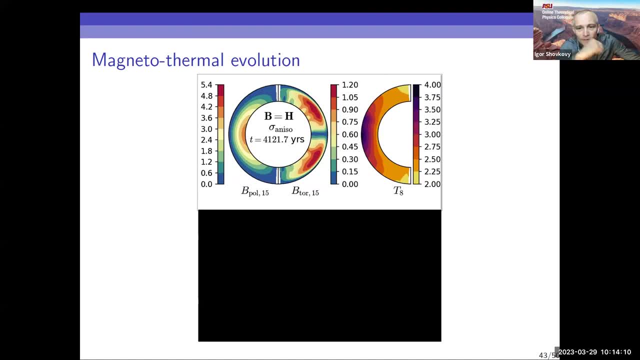 And I'm sort of confused by that. So, yeah, the simulations I have seen, like I've, yeah, when I've seen these, they do tend to say that it's actually the equator which gets hotter. So, naively, again, maybe I'm missing some important physics. 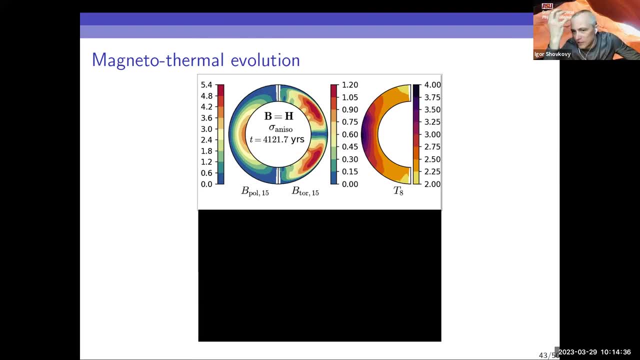 but naively. I know that the source of the heat is in the interior of the star, where it's the hottest, the densest and everything, Yes, And then in the magnetic field. I know that the parallel component of the conductivity in the directional field is typically much larger. 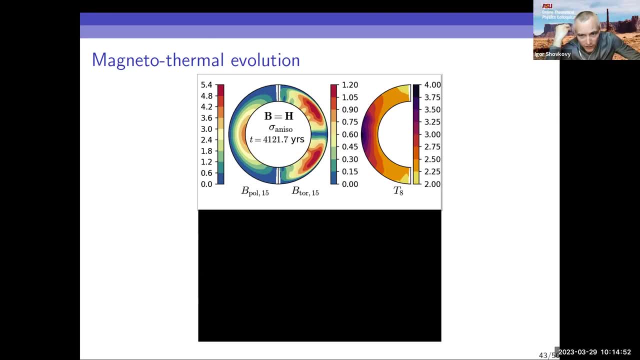 than perpendicular. So that basically opens kind of like direct sinking mechanism of the heat through the magnetic poles, not to the equator, And that's where I would expect the hotspots as a result. Is there something wrong with that argument, Or is there? 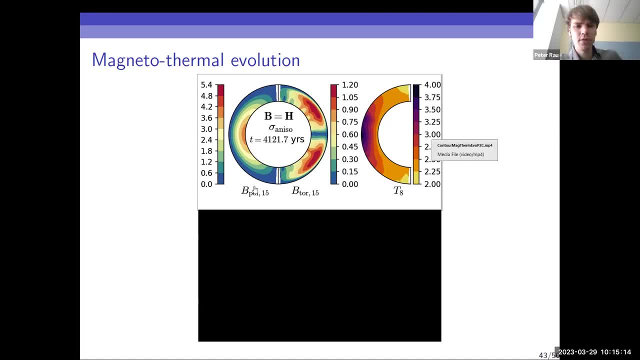 is there something else assumed here? Yeah, I mean if we look at earlier times. So I don't think no, I think OK. one of the things which is I think it's different in my calculation is I do not assume that the field is emerging from the star. 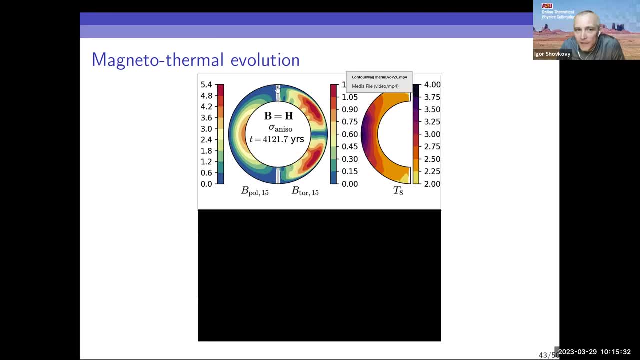 So if you look at like, Oh, I see that the magnetic field is completely absent and basically that heat is coming to your outer layer. Yes, Yes, Yes, Yes, Yes, Yes. This is like a layer to this shell, basically uniformly from all direction of the. 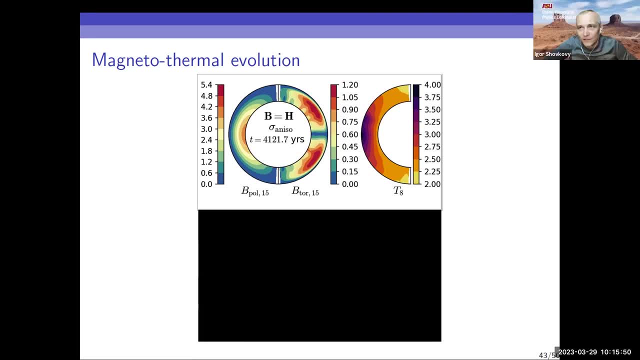 It comes uniformly from all directions of the core, Definitely, yes, I see, I see, I see, OK, OK, And so it's like This invalidates what I suggested, but I still think in a real star the heated hotspots should be. 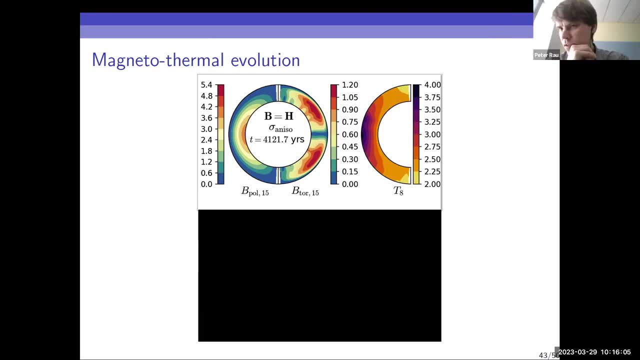 shouldn't they be on the pole? magnetic poles You do get the hotspots, but I think that has to do a lot with also external heating too. I see, I see, um, so i mean i'm i'm not worrying about like i assume i am matching to like potential conditions.